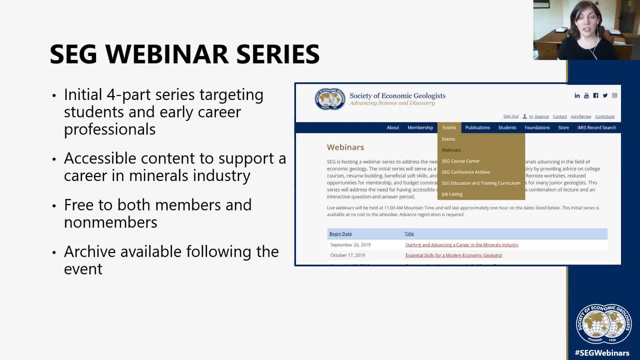 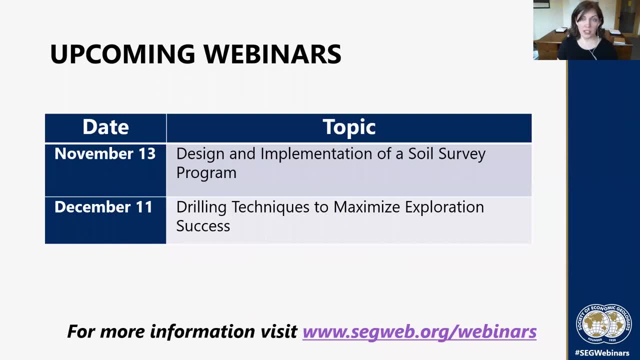 I encourage you to register for other upcoming webinars and details are available on the SEG website. Here's the list of the next events. I wanted to call out that there's a date change for the November. I had already called out that there's a date change for the November. 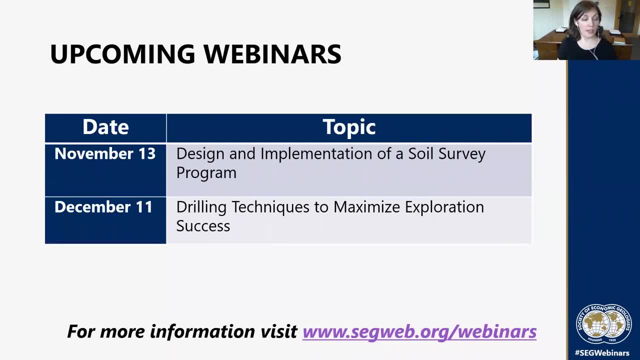 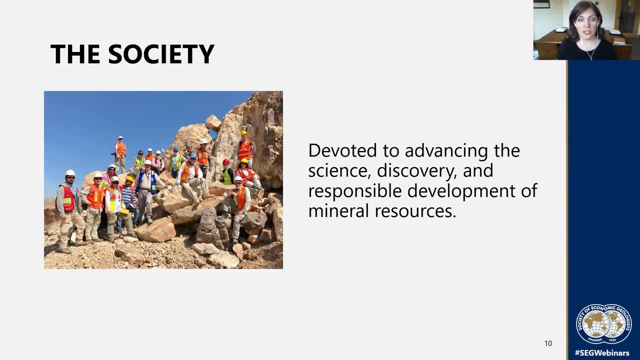 I'm going to go ahead and see if they are in. I'm going to click on the dr. Now I'm going to click on the December webinar. It's changed to the 13th And I will be sending out an email with that change following today's webinar. 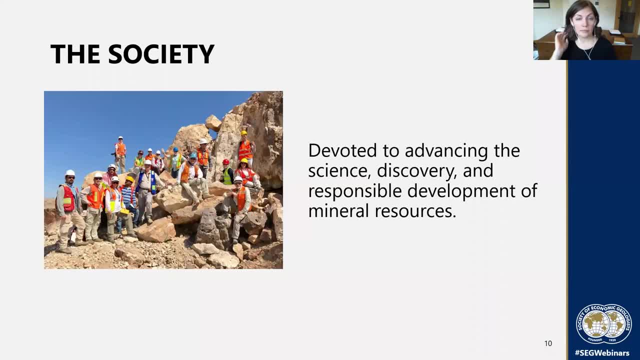 And with that, I wanted to take a quick poll just to see how many people who we have on the call today. Okay, All right, We have some great answers coming in so far, and I'll just give it a few more seconds before. 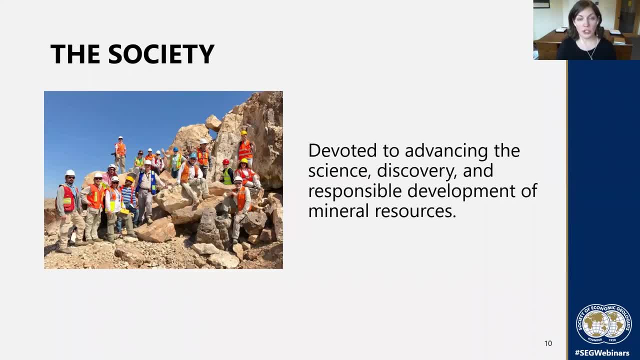 showing the results, So hopefully everyone can see the poll on their screen right now. Just asking if you're a member and where you're coming from. Okay, I'll give it a couple more seconds and then, all right, let's see what we have. 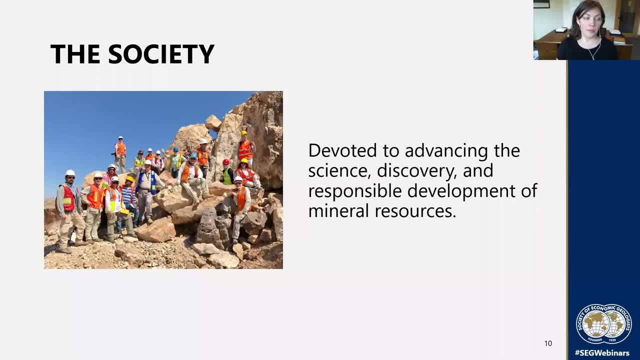 And I will share the results with everyone. So great. Most folks here are SEG members, but there's a fair amount who are not. A lot of individuals are coming from industry and we have a wide range of experience level here. Okay, 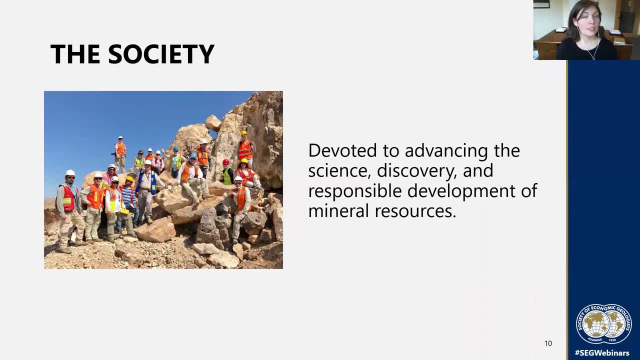 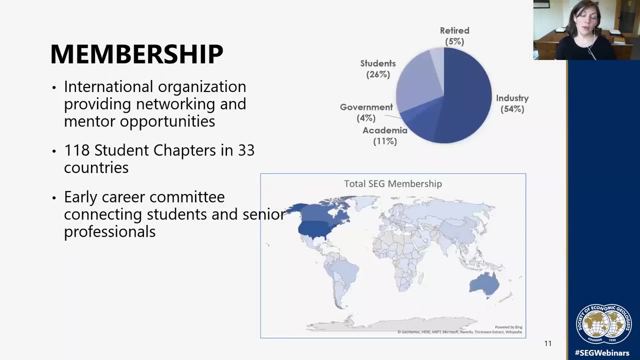 So for those of you who might not be familiar, but it seems most of you are, SEG is a society devoted to advancing the science, discovery and responsible development of mineral resources. We're an international organization with members all across the world, predominantly in North. 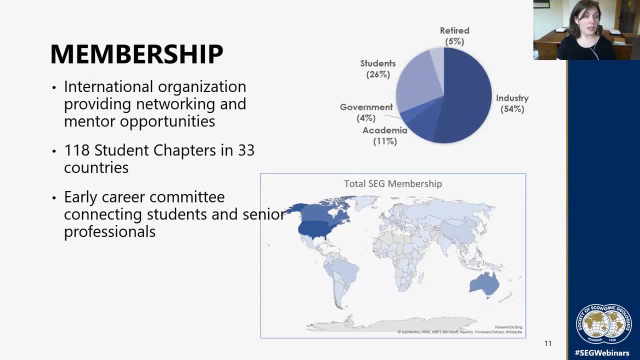 America and then a large portion in Australia as well. We have 118 student chapters And we have early career students And we have a career committee connecting students and senior professionals, And this just gives an overview of where our student chapters are at the moment. 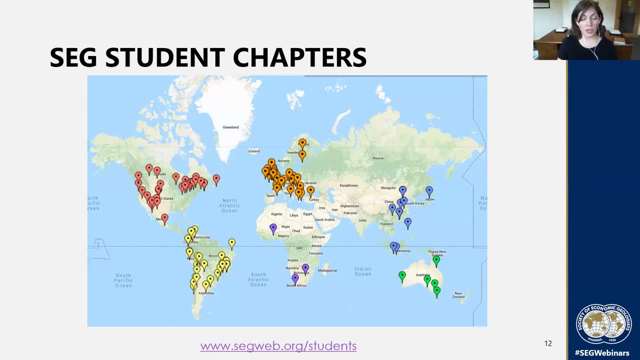 If you are interested in finding out more about a student chapter or how to start one at your university or college, you can go to the website segweborg slash students to find out more. And with that I will turn it over to Benedict. 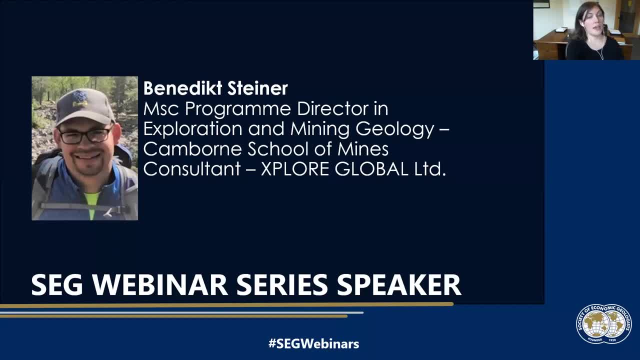 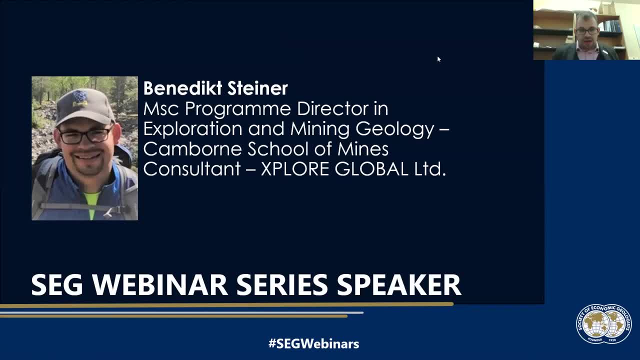 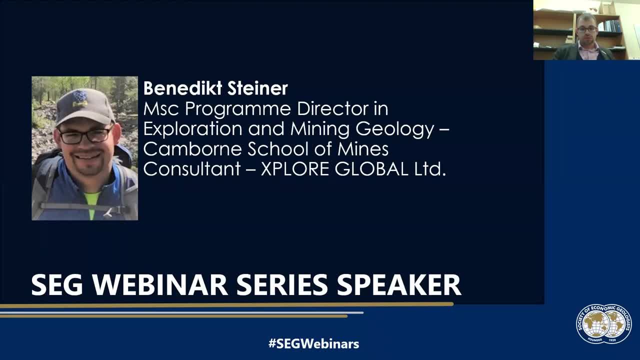 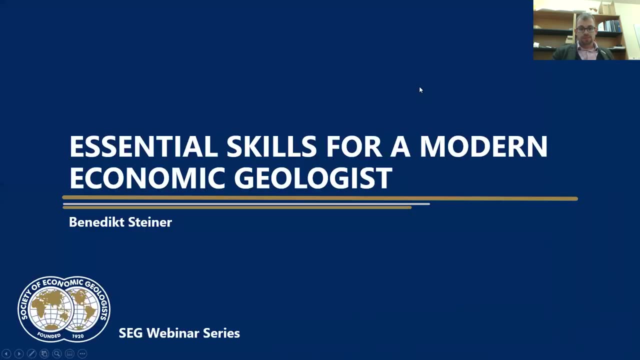 OK. So I think, Deanne, if you could move the slides, it doesn't seem to work here. Benedict, give it a try again. I'm going to close this. Yeah, I think it's better if you move it, please. 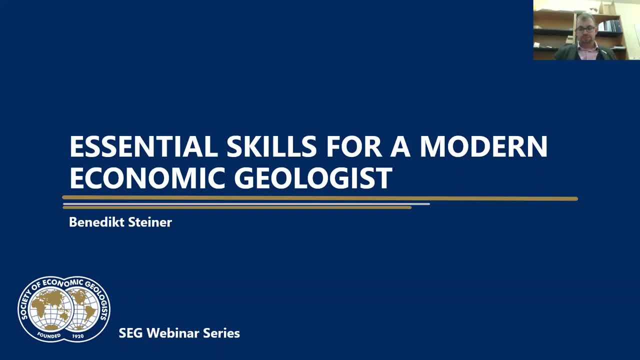 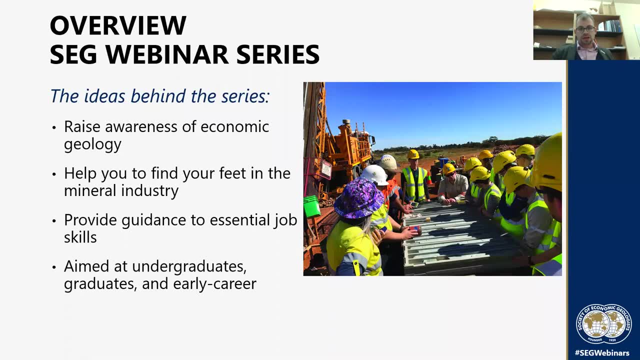 Okay, Yeah, Right. So sorry for the short delay And again, welcome to the second webinar in this series. And we originally had the idea to come up with a number of educational sessions on the topic of economic geology, With the aim to raise the awareness of economic geology and especially help you- and I mean by that early career professionals and graduate students- help you to find your feet in the minerals industry. 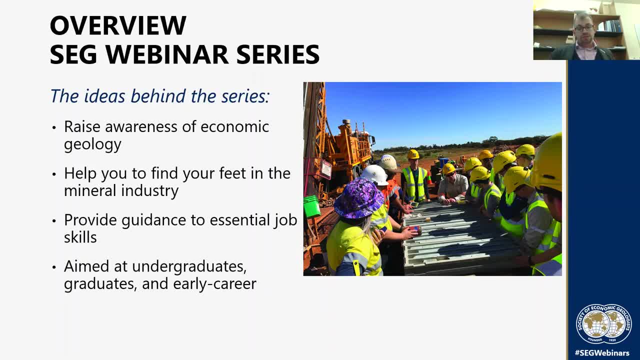 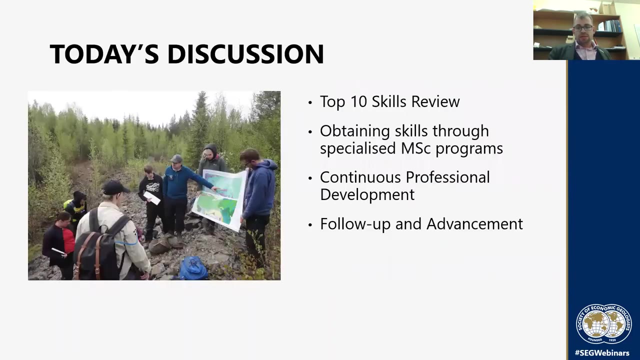 We would also like to open up this to provide guidance to essential job skills that are really needed if you're working, If you're working in mineral exploration, mining or related fields- Next slide. So today we are going to look into the top 10 skills that I believe are really critical in the minerals industry. 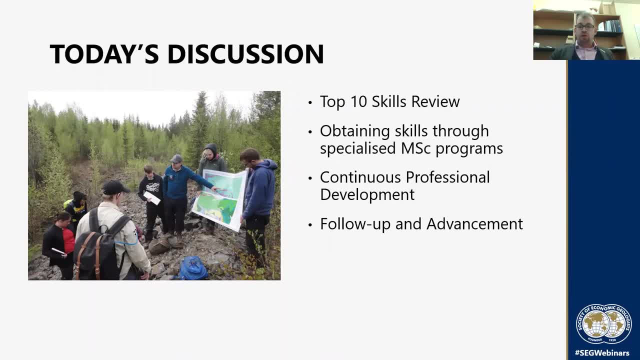 We're going through them and I explain to you a bit more what I believe geoscience graduates or early career professionals, what skills they should develop. Following this, I will present a few ideas and explain how these skills can be obtained through practical work experience or by studying specialized MSC programs. 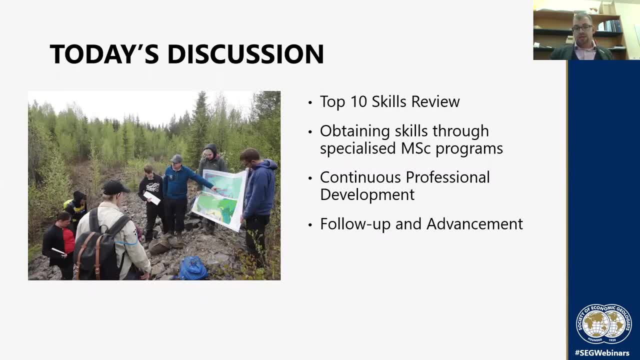 And I will also explain how these skills can be obtained through practical work experience or by studying specialized MSC programs. And I will also explain how these skills can be obtained through practical work experience or by studying specialized MSC programs. And for the professional members amongst us today, 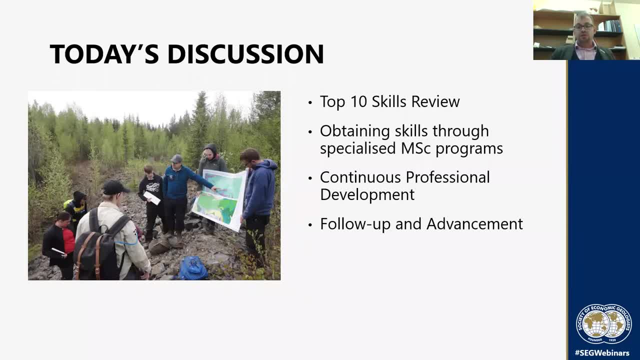 I also will give you a couple of ideas how to actually make use of the so-called CPD- the continuous professional development- to help you advance your career in the mining industry. I also will give you a couple of ideas how to actually make use of the so-called CPD- the continuous professional development- to help you advance your career in the mining industry. 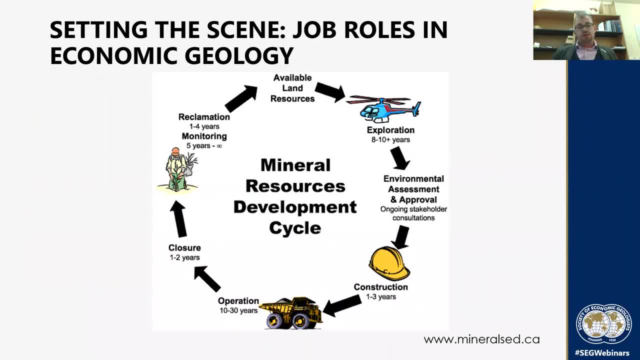 so last webinar, we have set the scene already, but just for those who didn't manage to attend, i quickly summarize the key points once more. the mining industry actually is quite a that, the right offers, the right employment opportunities, and all of those can be placed along the 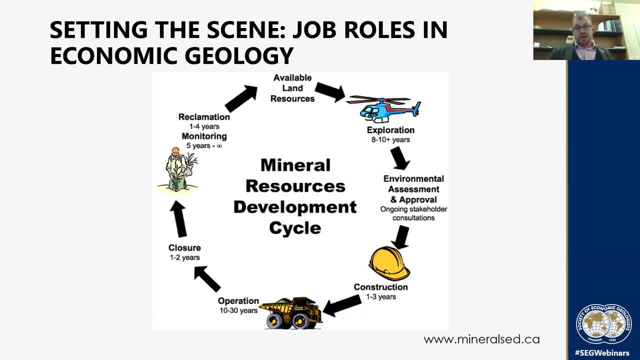 mineral resources development cycle, if you like, and this development cycle describes all activities that are related to mining in the minerals industry. now, usually that cycle starts off with the exploration phase. that's where geologists go into the field and aim to find mineralization and evidence for an economic and mineable ore body. 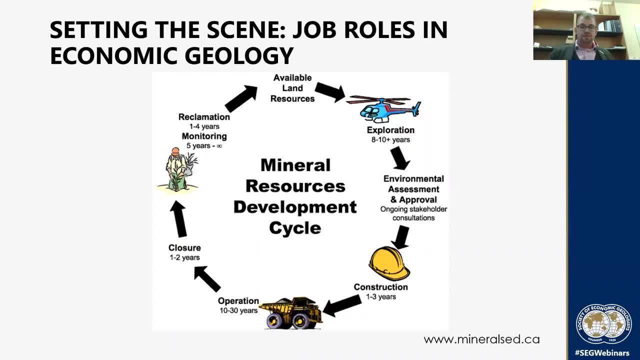 following: this usually have environmental impact assessments and approvals, which is granted by by the government or environmental authorities. if, if those permits are all granted, the mine construction can usually start and all deposits are mined for a number of years and that really depends on the size of the the ore deposit. usually when these operations close down or are near the end. 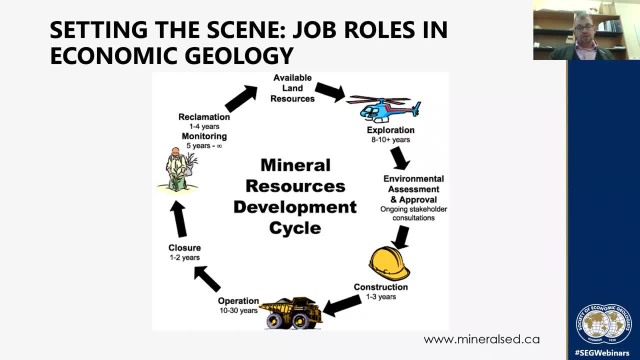 of their lives, a life cycle. we have the so-called rehabilitation and closure process, where the so-called- you know, the disturbance of the environment that's been done by the mining is attempted to be reclamated. I'm sorry, I'm sorry, I'm sorry. 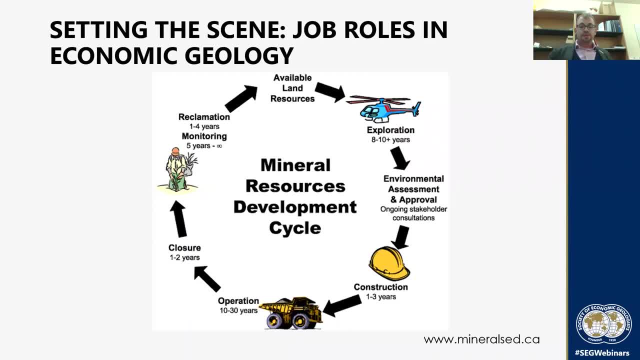 Now, all along this is mining development cycle- you will find job opportunities or career opportunities as a geologist to advance your career and, as I said today, we're going to look into the top 10 skills that I believe you should look into or you should acquire if you would like to advance your career in. 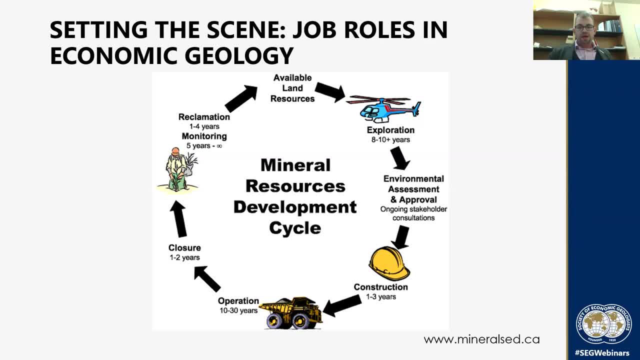 mining, and I think we have. before we start off with these skills, we have a short poll coming up, Dianne, if you could kindly move them in right, so I would like just like to ask the audience what skills you think are the most essential for economic geologists. do you think project management and organization is is key to 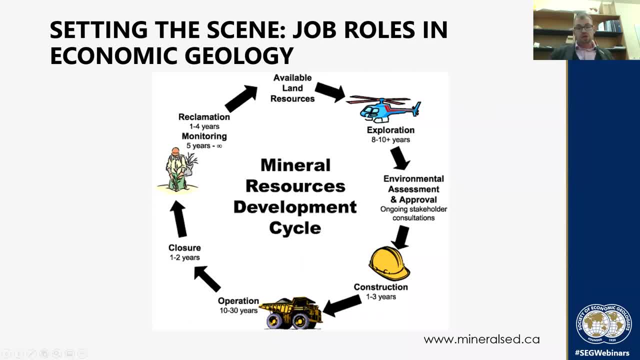 a job in in mining and exploration, or do you think communication skills are important, or actually the technical knowledge? so the the pure geology aspects, although you believe soft skills and problem solving skills is well of importance. so please take your choice and let's take a look what. 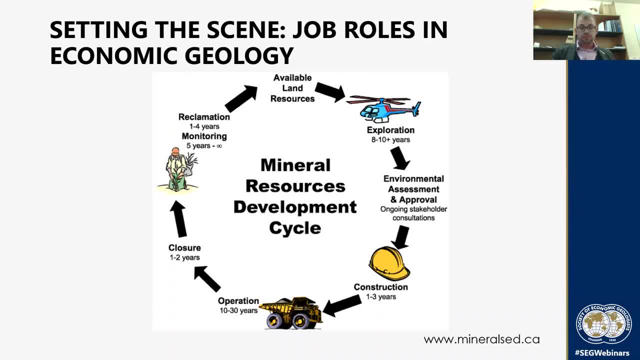 what the audience thinks. let's take a look and see how frank i think this was number one. okay, um the end. maybe you can show up the results of um this quick survey. great, so we seem to have almost um the results of this quick survey. great, so we seem. 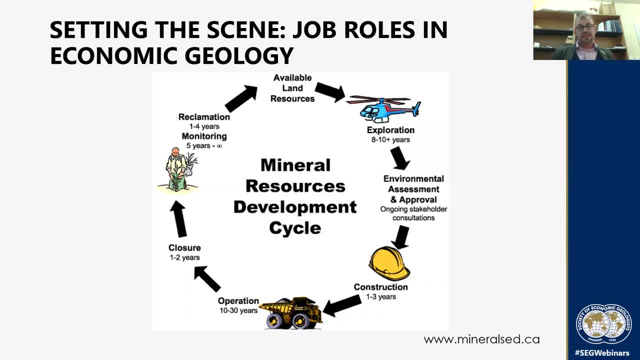 of the audience believes that technical knowledge such as geology and fieldwork is. those skills are critical in carrying out a job in mining and exploration. and then we've got about 33% believes that problem-solving and creative thinking is is the way to go. so that's, that's very interesting, so I 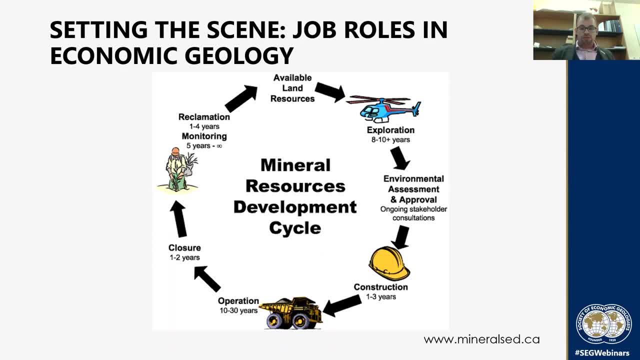 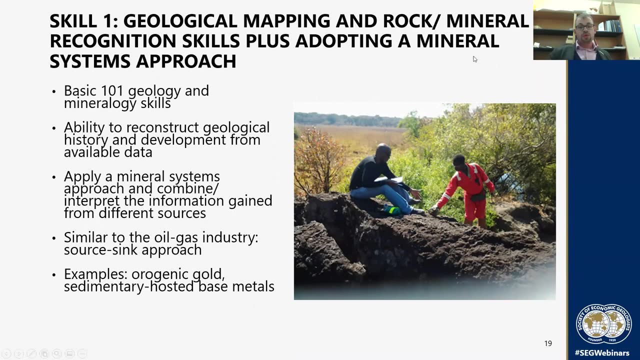 suggest let's take a look at what, if that, if that matches up with with what I'm happy going to present, all right, um, let's move to the next slide and start straight off with skill number one. well, I believe that in mining exploration, geological mapping and rock mineral recognition skills is absolute. 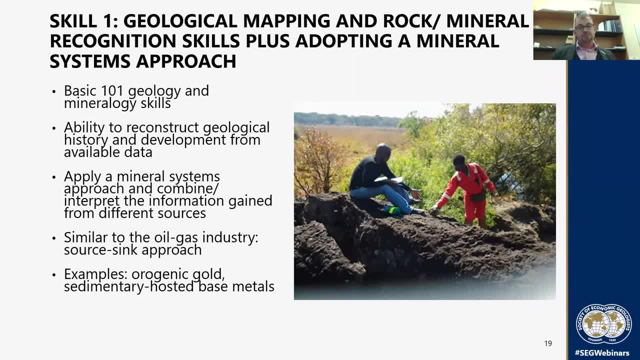 guarantee key plus adopting a mineral systems approach. so in a way, that sort of reflects the nearly 50% of you that have voted for the technical skills that are of importance. so what do I mean by these geological mapping? well, it's, of course, very obvious that if you are going to look for, look and mine, all deposits in 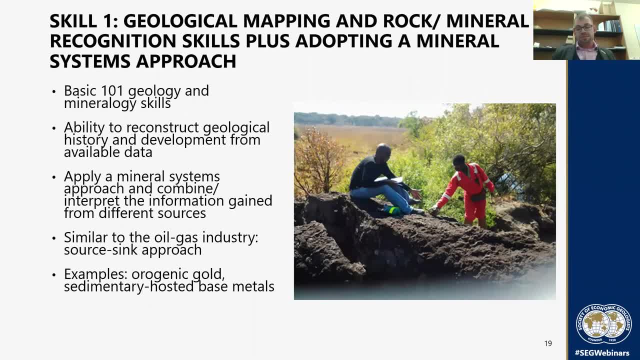 the geological mapping theCUBE, know how to produce geological maps with the knowledge and understanding that geology is key, but I really believe that you need to. you need to acquire the, the basic skills that you learn in your first University years. those are the really the key ones that will help you to be. 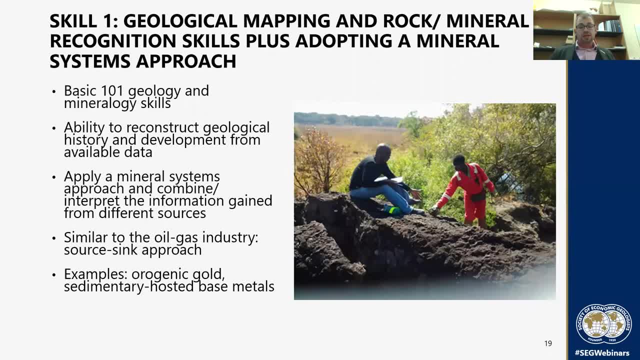 construct geological history and development from the available rock and geological data that you acquire in the field, And that is critical, as we in mineral exploration and mining we would like to understand how ore deposits form, And here the concepts of the mineral system approach analysis really comes into play. 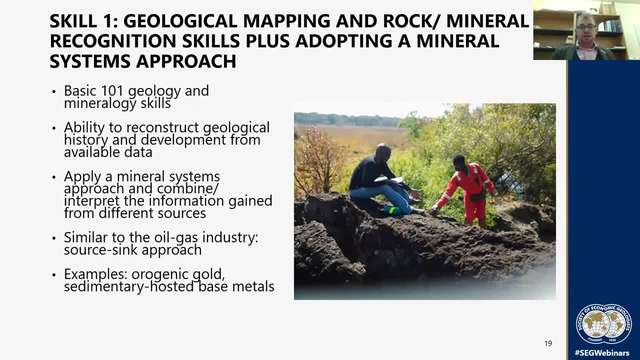 So mineral systems analysis aims to combine and interpret information gained from different kinds of techniques and sources, such as geophysics and geochemistry, And it's quite similar to what the oil and gas industry has been doing for decades. And mineral systems analysis tries to put an ore deposit into perspective. 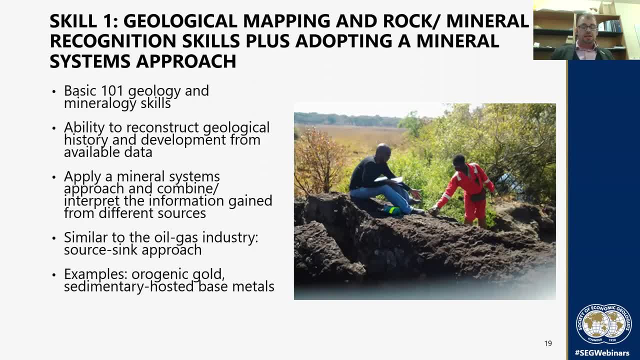 So you would like to analyze where's the source of mineralizing fluid, how does it travel to the host rock and how is it deposited there and forms actually the accumulation of economically interesting minerals. Now, this understanding is important in order to predict the occurrence. 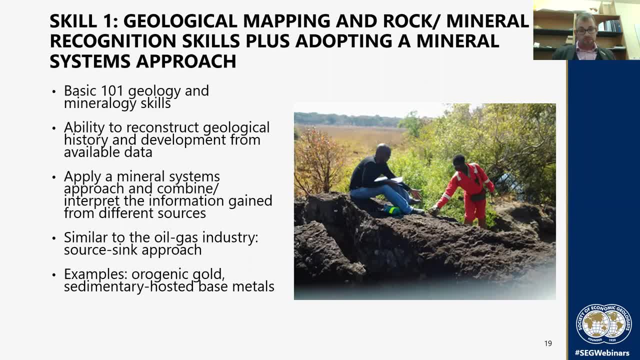 Okay, And the location of all deposits, And this can, of course, be applied to all sorts of mineral systems. I'm just giving two examples here. I've listed orogenic gold deposits and sedimentary hosted base metals. Now in orogenic gold deposits. those of you who worked in the sector you know that orogenic 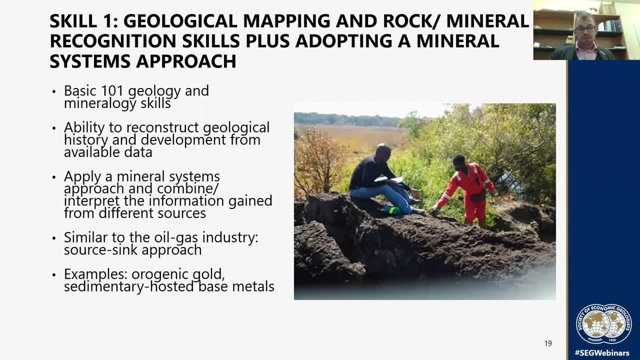 gold has a very, very strong structural influence. Okay, And it's also very important to understand that the deposits are usually found near regional shear zones and along these shear zones you have these mineralizing fluids traveling and then deposited in mafic or graphite rich host rocks. 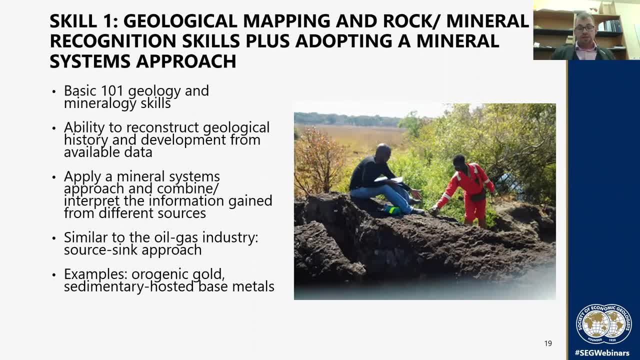 Now understanding these different structures and the structural development of an area, along with the chemical process, Okay, And the chemical processes that take place in the host rocks. that's, of course, very, very important if you screen large areas for prospective structures and deposits. 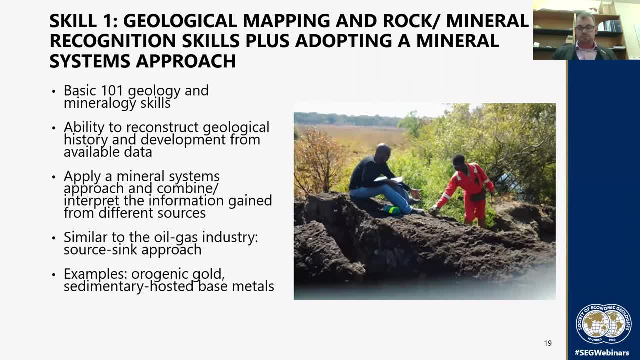 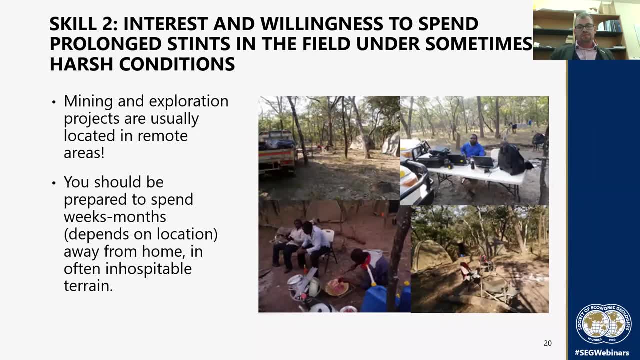 If we move on to skill number two, I believe that here a bit of- yeah, a bit of- a technical soft skill, you should have definitely an interest and you should show the willingness to spend prolonged stints in the field under sometimes difficult conditions. let's say, 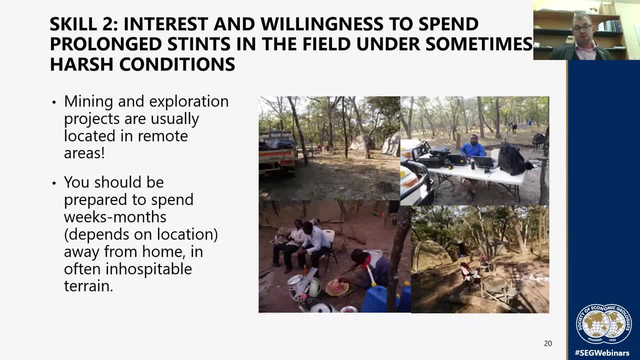 If and when we are looking for new deposits or actually mine them. nowadays it is in quite unaccessible regions, And I'm just quoting excitement. I actually I have an example which is more of a comparison with the examples of Northern Canada or Central Africa or the Australian Outback. 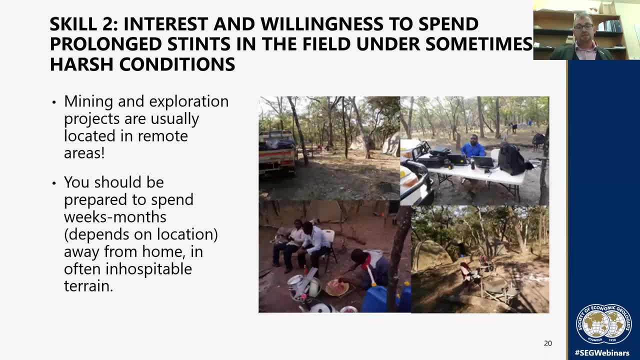 These areas are probably quite under explored, but that's exactly what makes them attractive to mining companies And if you're working as a geologist in these regions, you would probably have to adopt through the thoughts of that You will be spending quite a considerable time away from mining, from mining systems. Etc From home or from your base locations, and then that, depending on the location, can be ranging from weeks to months. Alright, so I know that If you're working in Africa, usually spending their weeks or up to three months, while in other parts of the world, you 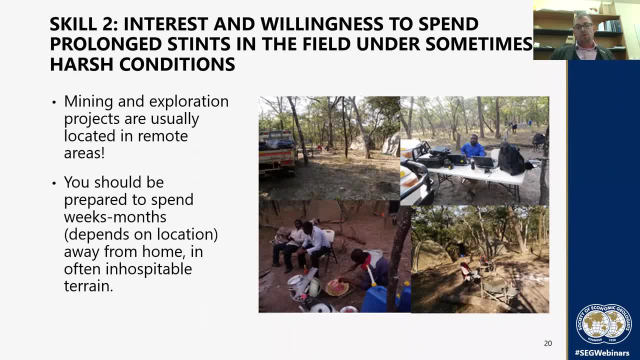 Probably spend just a week in the field and come back Now. Why do I mention this? Well, I, I think not everyone is comfortable in living such a lifestyle and being able to- Yeah, being able to- spend long periods of time under such conditions. 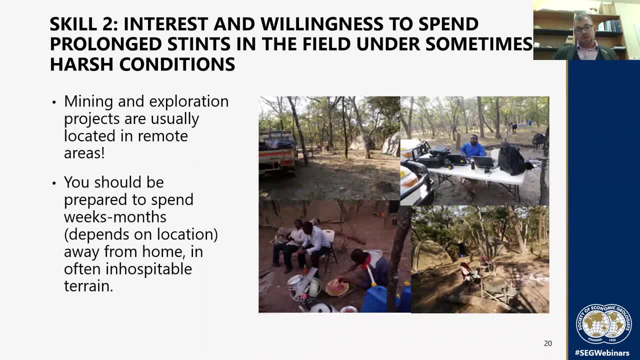 so if you, If you're still deciding whether this- Whether economic, geology or mineral exploration- is the right thing for you, I believe that you should consider this, this point here, carefully, And I guess what helps is always speaking to colleagues or industry contacts that you know Who have done this kind of job already and can tell you about. 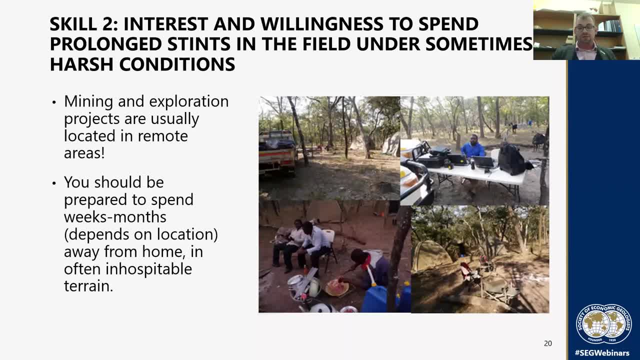 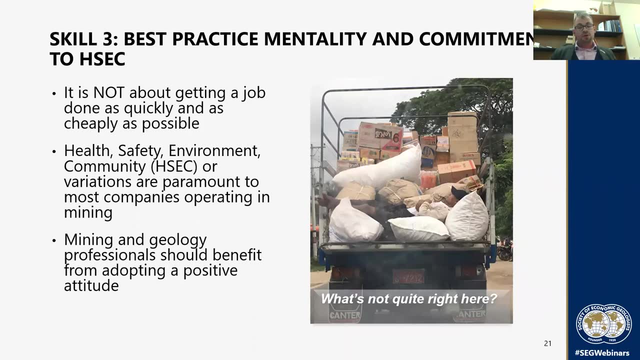 the different social aspects of of such broken lifestyle. If we move on to skill number three, I think here's a very important aspect actually. just take a look at the photo on the right here that's. that's a photo I took last year when I was on field. 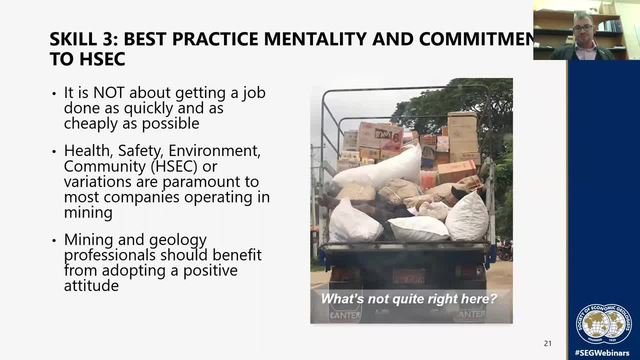 work in in Southeast Asia. and of course, you might ask yourself, yeah, what's not quite right here? and there's some in this photo. well, there are a number of things that are not quite right here, but I think all of them go back to the common aspect of health and safety. now, what I'm using here, HSE sees, you know. 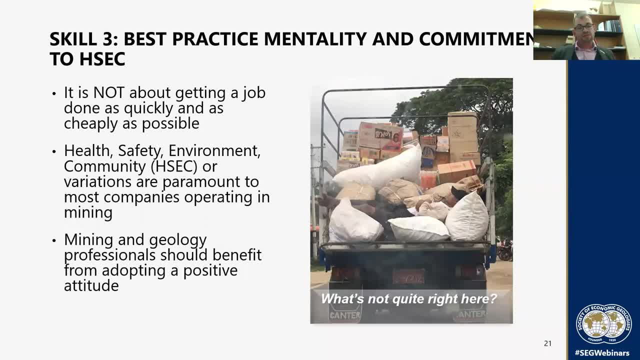 that depends on the company you're working for, but it usually stands for something like health, safety, environment and community, and these aspects are paramount, really paramount, in the mining industry nowadays. so it's not just about getting a job done quickly and as cheaply as possible. well, that's. that's a common attitude I've 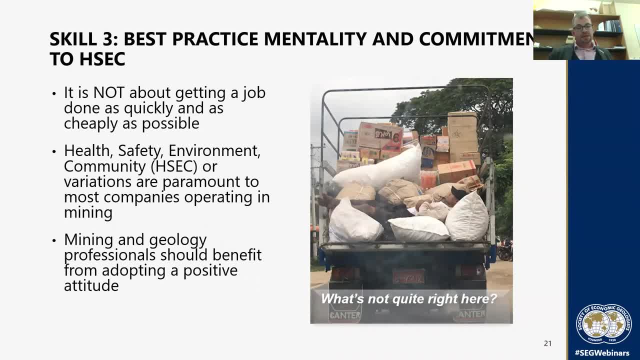 seen, but really nowadays, you will quickly realize that the mining industry has strict norms and regulations and most companies are that are operating in in the minerals industry, having their own health, safety, environment and community standards. I believe that mining and geology professionals should really adopt a positive attitude towards towards this aspect. so the aim is that you know you. 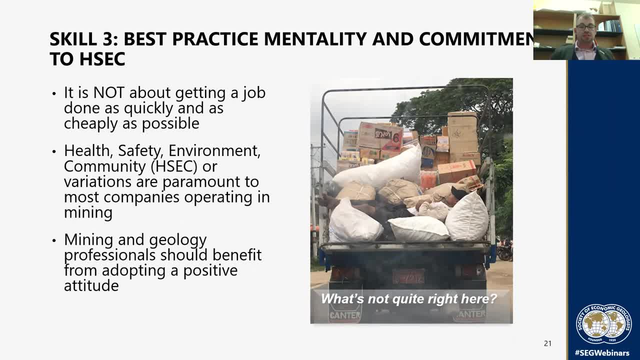 go on a work stint and you return safely and without any harm. equally, that applies to the environment or the communities, the community sector you're operating in. So what I want to say by this is that the social and environmental aspect is extremely important in mining. That's usually not something that's been taught at. 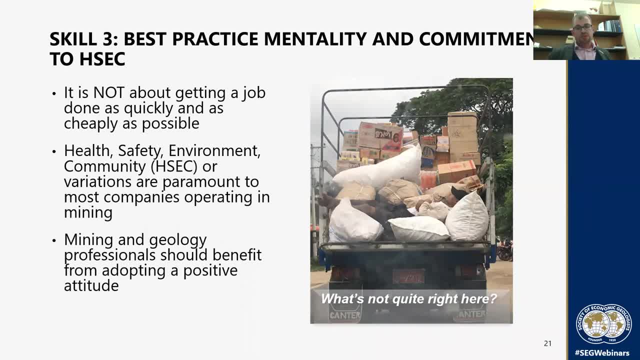 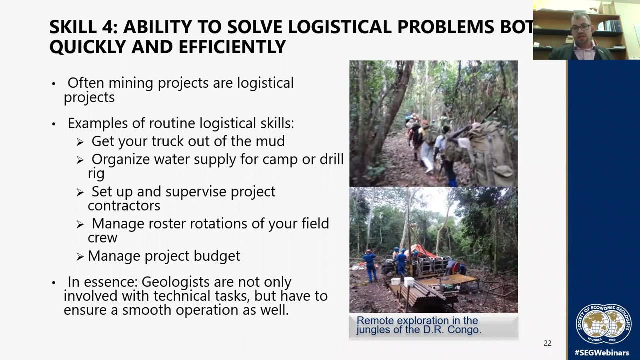 university, but I would suggest that weeding into this aspect could be quite beneficial to you acquiring the awareness or the skills to succeed in the mining industry. If we move on to skill number four, you can see here on the right-hand side, these two photos. here They've been taken. 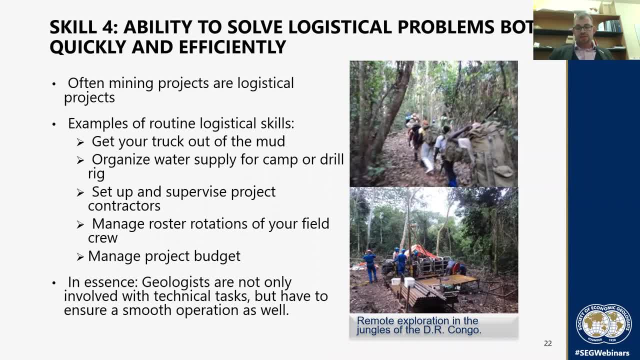 from a remote exploration project in the jungles of the Democratic Republic of Congo. You see there that on the top photo everything is logistically being carried by hand in the jungle. There is absolutely no access there. Even the drill rig on the bottom of the jungle is being carried by hand. 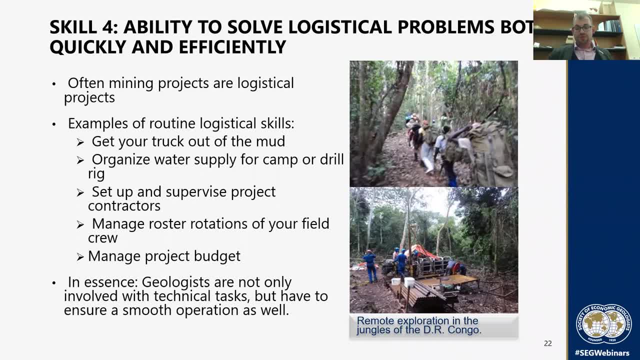 The top photo has been hand carried through the jungle. This is, of course, quite a logistical challenge and problem if you operate in remote areas. Now, often mining exploration projects have a huge logistical tail. What it means is that it's often quite a challenge to organise. 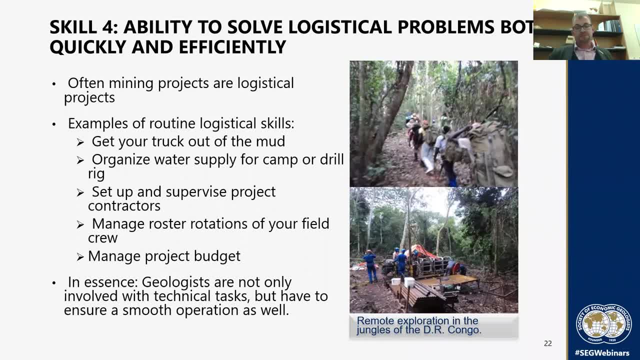 field programs and field projects efficiently, and what i learned by in my career in the mining industry is that being able to to to solve logistical problems and acquiring these logistical skills is really, really important in order to actually carry out your normal job, which is geology. so i'm quickly giving you a couple of examples of what logistical skills or say: 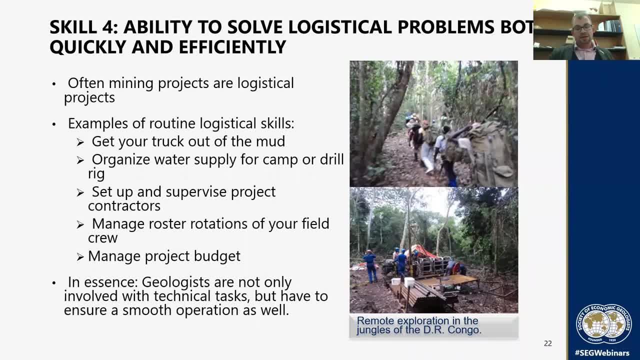 situations you might encounter when you, when you work out there in the mining industry. so first of all, i mean some of you who read this, you probably have experienced this already, but those, those points are just some of the classics. i think so. for example, in such remote areas, if you're driving these large four by fours or trucks, it's almost guaranteed. 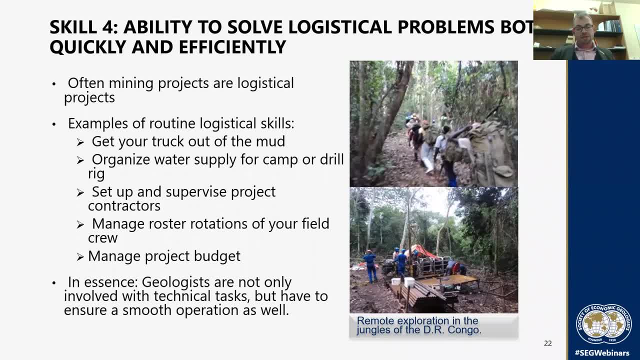 that you get stuck in the mud at some point, especially in the rainy season. now, getting your truck out of the mud is a is quite a sophisticated skill, especially if you haven't driven those large vehicles before. so i think that is something you will quickly learn if you're, if you're doing. 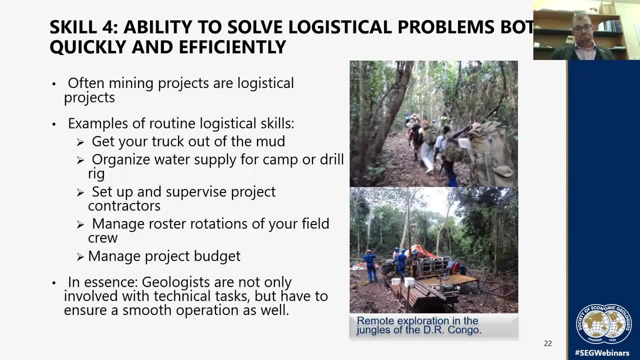 remote field work. another um. another skill i learned myself in the field was, for example, to organize water for, you know, for field camp or for drill rig. now, you know, diamond drilling rigs. they consume nowadays up to 10 000 liters of water a day. now, if you're operating in a desert, 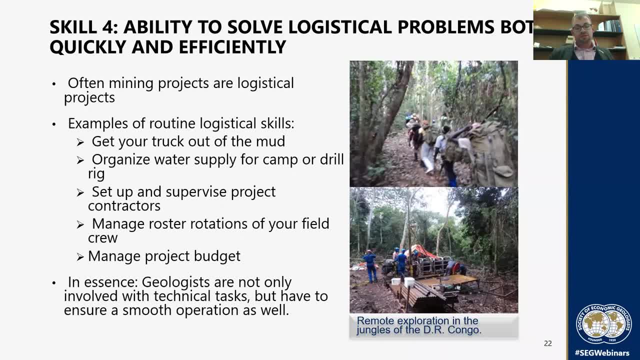 where would you expect to be in a desert and what would you expect to see in a desert? you get 10 000 liters of water every day from now. um, that's a very interesting, um interesting question. do you truck it in from somewhere else or do you drill a borehole and extract the water? 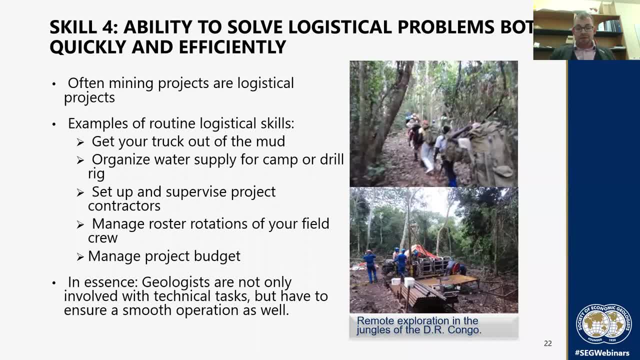 from this borehole. that might have some environmental implications. um, this is, of course. yeah, this is a very important aspect. without water, it's very difficult to carry out any diamond drilling um. point number three here is set up and supervised project contractors. every exploration project or mining project makes use of a whole range of contractors. 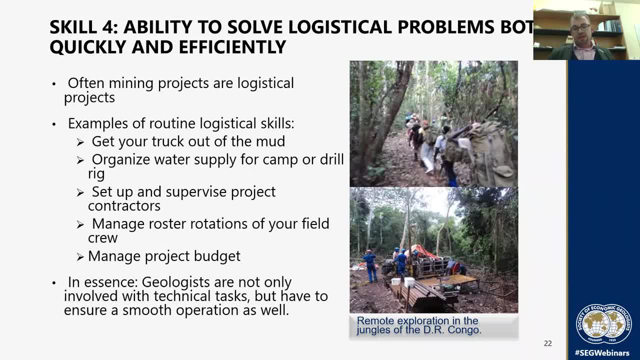 whether they're drilling operators or, um, um first aiders, or people supplying procurement services to your, to your project- all of these need to be somehow organized and supervised, right? you, of course, want contractors to carry out a proper job. now, um, that's also something that's usually not taught. 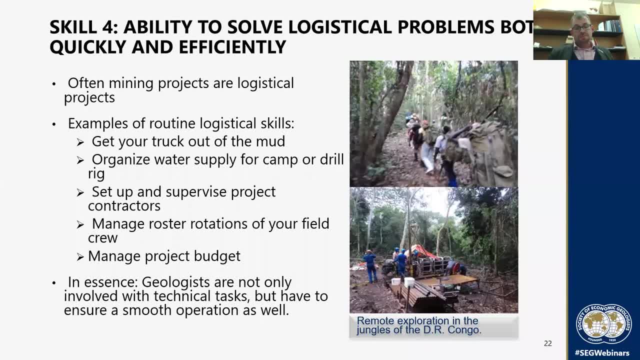 at university, uh, but really an important skill to to learn. so if you have the chance to um to start managing people and during vacation projects, or if you're a graduate geologist, uh, you may want to really get involved in this sort of um um area here if you're a bit more advanced. 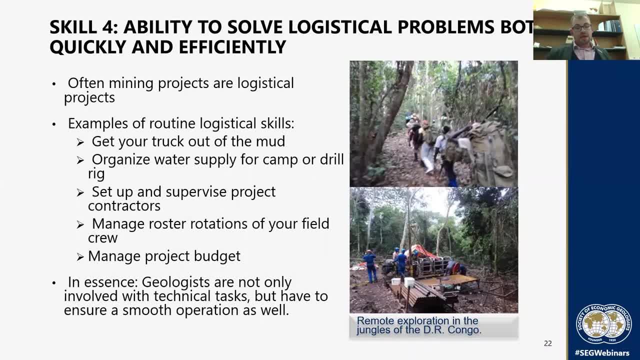 in the uh in in your career ladder, you may be uh managing the roast rotations of your field crew. so what? what do i mean by that? usually project managers. they manage, um, how people move in and out of uh of a field project and whether they drive in or they fly into a 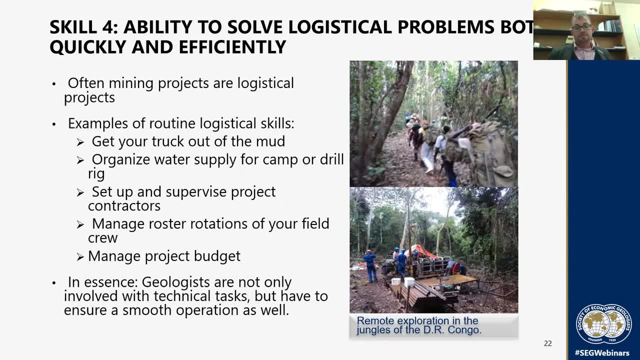 into a certain location. all of this needs to be managed and if you're having 50 people on your team, it can be quite a challenge to accommodate everyone's needs and wishes and also fine-tune this with any flights or transport going in and out of the project side, and a very another. 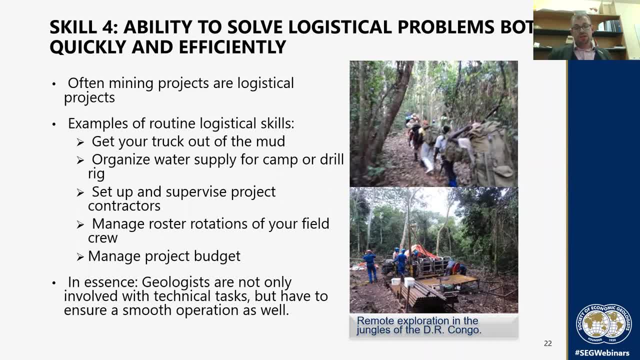 very important aspect is to manage project budgets. now, um, it's, it's usually the case that uh budgets and mining exploration are usually quite tight, so you can't, of course, overspend um money on on a project, even though that sometimes happens. but it really requires careful, um careful, understanding of where money is spent. 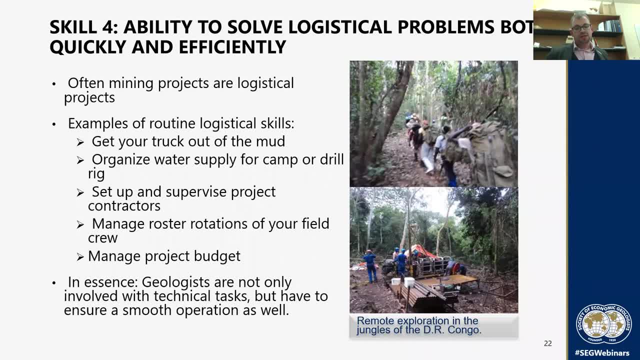 and how money is spent, and that's a key skill in in running such projects, especially if they cost lots of money, like on the right hand side in these photos. yeah, so in essence, what i'm trying to say here is that geologists are not only involved with technical tasks, so they're not just going out and 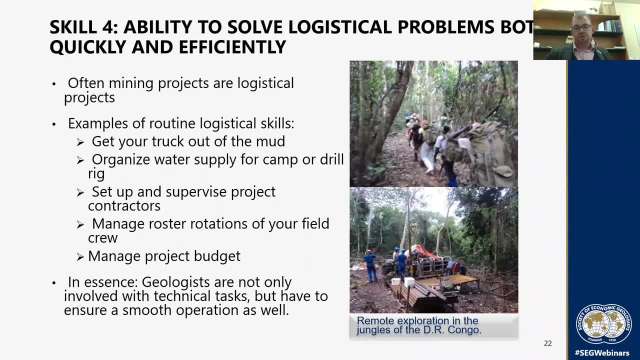 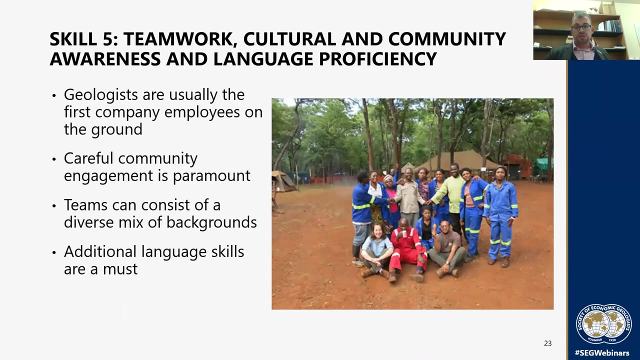 mapping an area, or collecting soil samples, or drilling and obtaining drill samples. really, um, your role as a geologist will often involve logistical issues and you have to deal with them rather quickly and efficiently in order to ensure a smooth operation of, of of um of your project. okay, um, let's move on to skill number five. 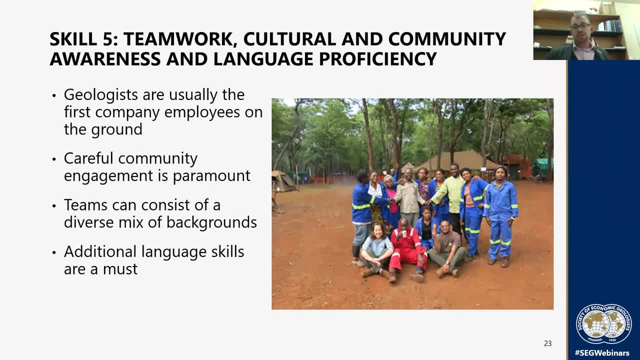 teamwork, cultural and community awareness, as well as language proficiency, efficiency. i'm sure um many of you who already spend some time out in the field, uh, working with people from all around the world, you will realize that mining is a very global business and it is not uncommon to have many different people from different cultural backgrounds. 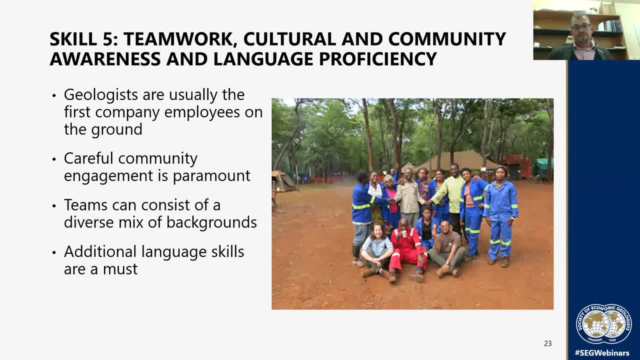 speaking different languages and having different habits, and habits on site. now, this is especially true if you work in places like asia or south america or africa, and as geologists, you're usually the first company employees on the ground, if you like. so the the local population. they will see the company through um, through how you, how you act and how you behave. 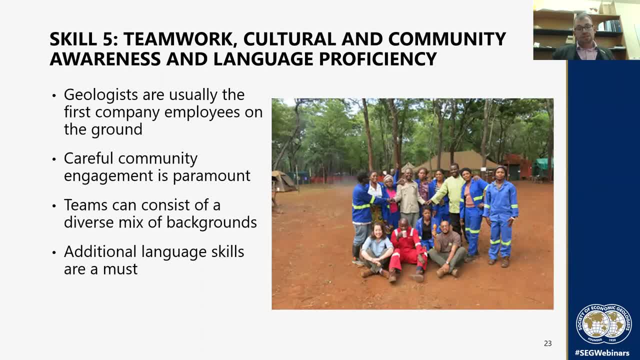 so careful community engagement is absolutely paramount in in the mining industry. um, and as your team can consist of a diverse mix of backgrounds, that can lead to quite interesting um team dynamics and in carrying out a job- importantly here as well- um additional language skills are really a must. 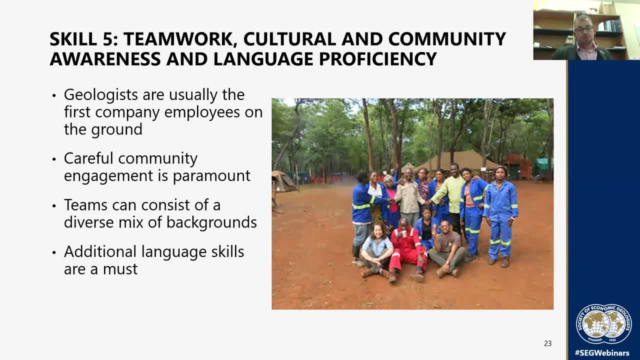 um, if you're, if you're working remotely on remote sites, um, and if you speak other languages than english, um, that's often a very great advantage to um to be able to liaise and communicate with uh, local people and even contractors. so i've had many times the experience that 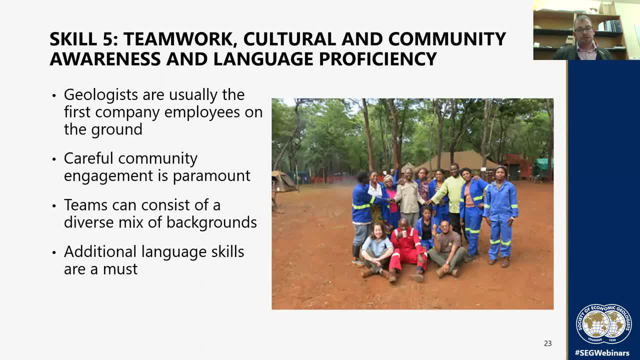 if you try at least to speak a local language, that people will very quickly warm up to you and accept you as a as a professional in the team, because that just shows that, um, you have the ability to, um, to fit into a different- you know a different- cultural background. 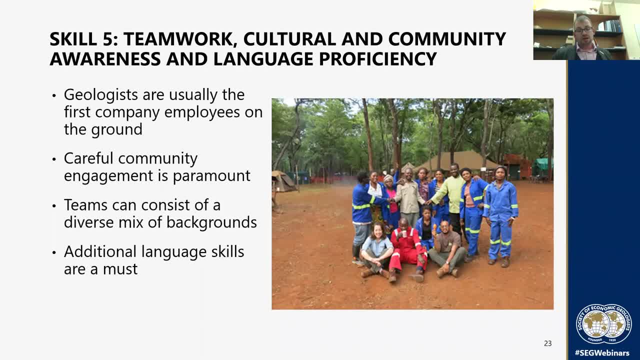 and community. so my recommendation uh to you is that um, learning other languages are there. it will really pay off over the long run. so you could think about learning spanish. you could think about learning french russian if you work in in more easterly directions, but also, of course, if 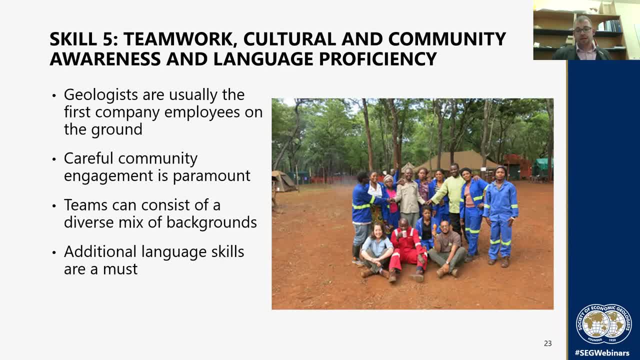 you work in areas where you have different tribal languages, like here in central africa, as you can see on that um photo on the right um, if you simply learn a number of phrases or words, that will open doors and um people will make you feel welcome very quickly. 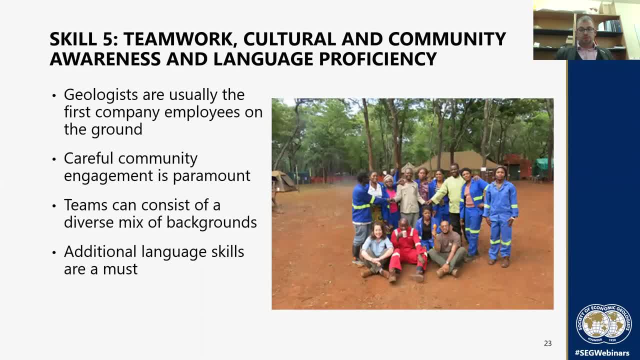 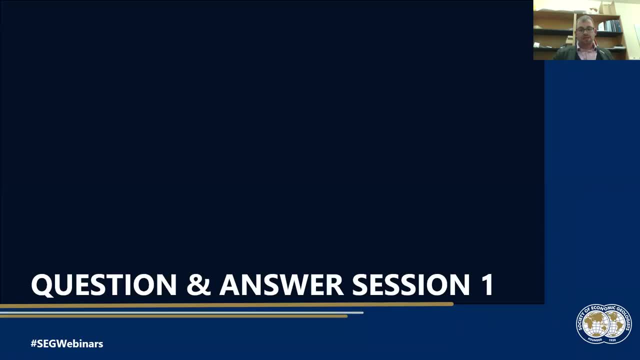 okay, on to the next slides. so, yeah, we arrive at um, our first question and answer session. um, let me have a quick look at the um question and answer sheet here. and we've got an interesting question here and um, the question is: uh, management skills is a must. 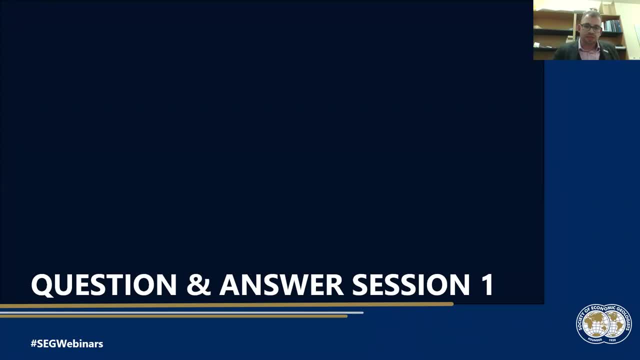 have. what about leadership? absolutely, leadership is is is very, very important. in my opinion, leadership and management go, uh, hand in hand. all right, so, um, if you're running a team, if you're, if you're managing a team, you of course need to, um, demonstrate it that you're a good leader. now there, 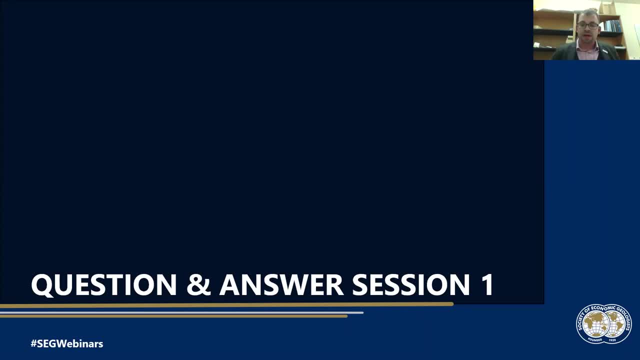 are, of course, different types of leaders out there, some who would like, who are very direct and very active. some other leaders are more passive and, let you know, other people carry out jobs, but really it is about developing these skills. um, that will, um, that will put you in front of people and allow you to, you know, be accepted, to run. 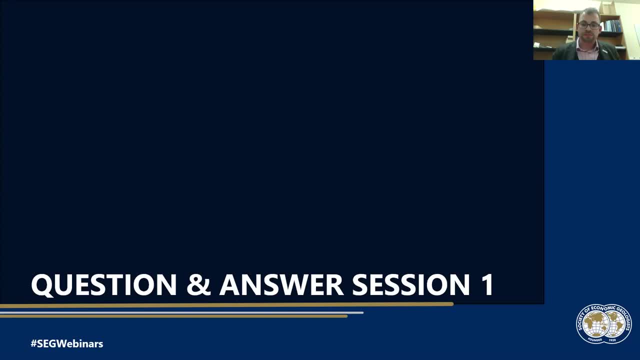 a program, run a project? one more question we've got here and someone is asking: is reflected light microscopy still relevant to teach at ESC geology level? now, this is a this is a very- yeah, very interesting question. let me answer it like that. I still believe microscopy is important in understanding rocks and 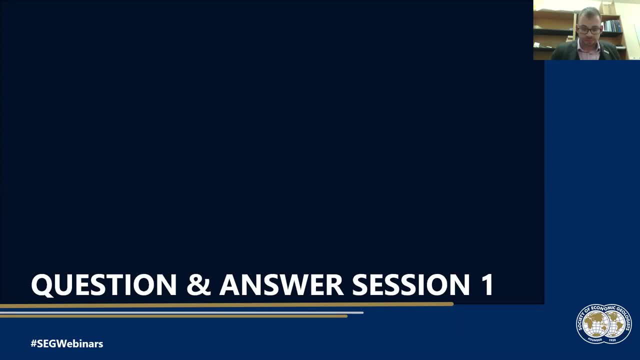 petrogenesis and mineralization suite mineralization suites, however, I have in my career in the mining industry, I've personally never used reflected light microscopy. if a question ever came up, it was either done by someone, by an academic at university or specialized consultant. so people may have different opinions about this, but I still believe. 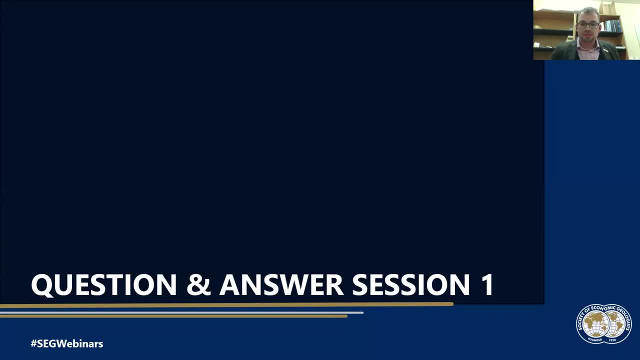 it's important that you, that you teach this and learn this at university. however, it needs to be clearly emphasized what the application of it is in in the industry, and that could be along the lines of identifying properties for geomaterial testing or process mineralogy. so if those, if those applications could be, 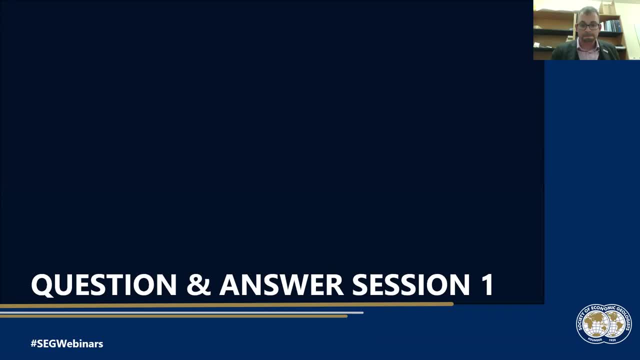 emphasized. that would be. would be fantastic, great. there's another question here: how was your change from oil to the mineral industry okay? well, maybe you've heard in my last webinar that I actually first worked in the oil industry and then moved into the minerals industry. so, if you like, I can quickly elaborate on this. 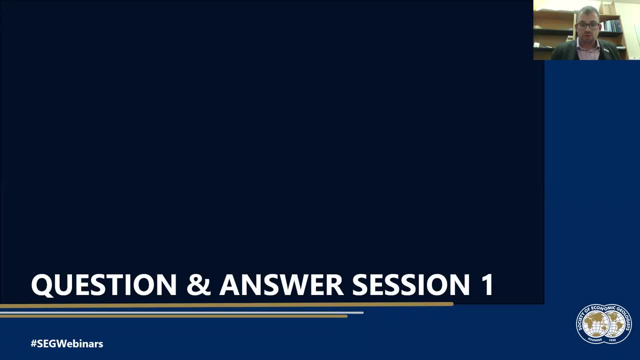 one. well, why did I change into into the minerals industry? well, for a simple fact that I really missed the fieldwork aspect in the oil and gas industry. I was sitting, I was sitting on a computer for a year almost and just digitizing well logs. now it might appeal to some people, but really, after University I personally 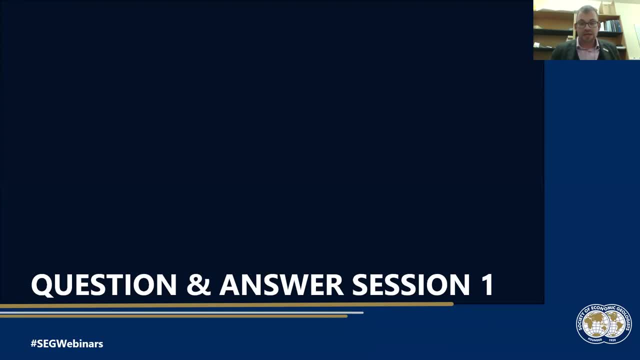 wanted to, to really get out, get experience, really apply my geological skills to two actual rocks and, in a way, yep, I definitely found this in the minerals industry. so in my opinion, this change was unproblematic. I did it very early on in my career, so I 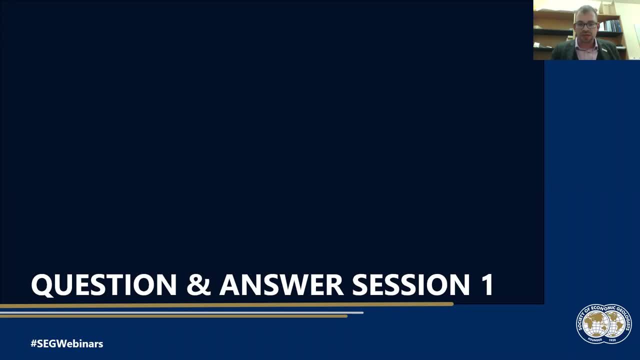 was not too deep into the oil industry at this stage. yeah, so I hope that answered the question. All right, I think we should move on. Thank you very much. We have one other Q&A session in a short while. Okay, Let's move on to skill number six And this. 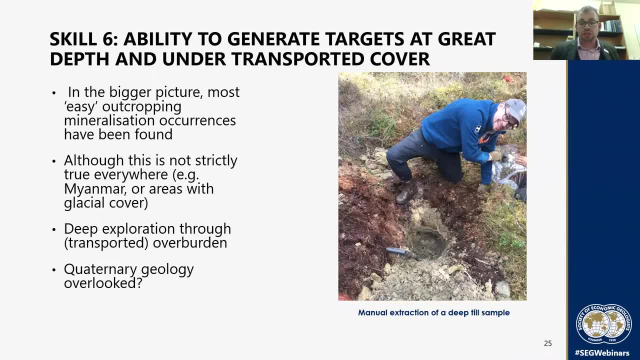 here gets a bit more geology Again. we've talked a lot about the soft skills and these management and logistics skills, but let's get back to some of the key geoscientific skills you will need Nowadays. it is well, it has been for a while, but it's even more important. 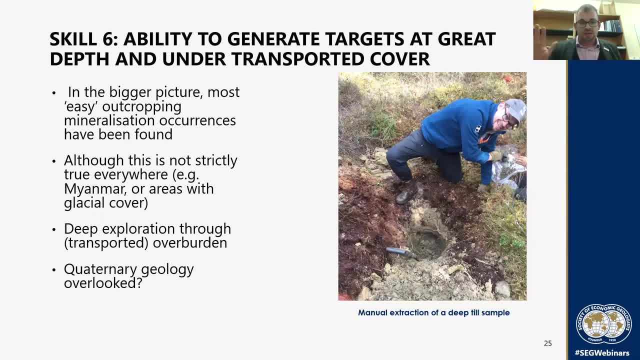 nowadays, with the depletion of the easy-to-find resources, It's very important to develop an ability to generate targets, exploration targets at great depth in under-transported cover. You can see me here on the right. I'm up in Finland and I'm digging a series of quite 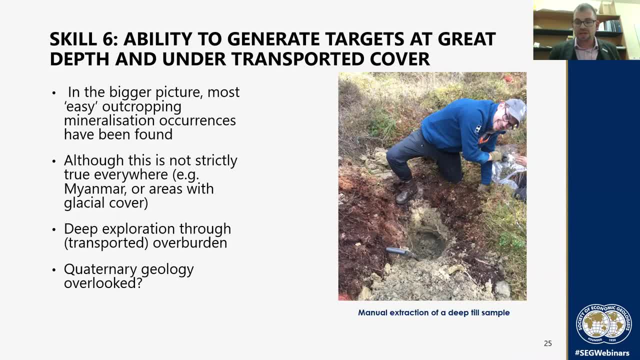 deep holes through glacial till. Maybe some of you know that glacial till is quite an interesting material as it has been transported for considerable distance. So if you just sample till you may perhaps actually find an anomaly. But it's been transported for a long distance and it's actually not sitting straight below. 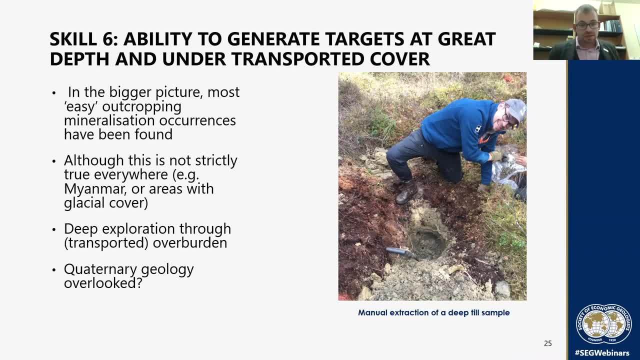 you Now, as I said, in the bigger picture, most of the easy outcropping mineralization occurrences they've been found. that's what's been said in most of the conferences nowadays. However, I believe that's not true everywhere. to be honest, I've been in places like Myanmar. 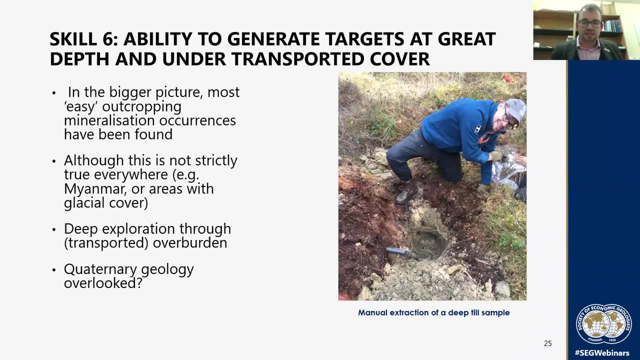 in Southeast Asia, in the Middle East, in the Middle East and in the Middle East, And I've been in places like Myanmar, in Southeast Asia and in the Middle East, And I've been, or in Scandinavia, a way of glacial cover where deposits are not deep In Myanmar. 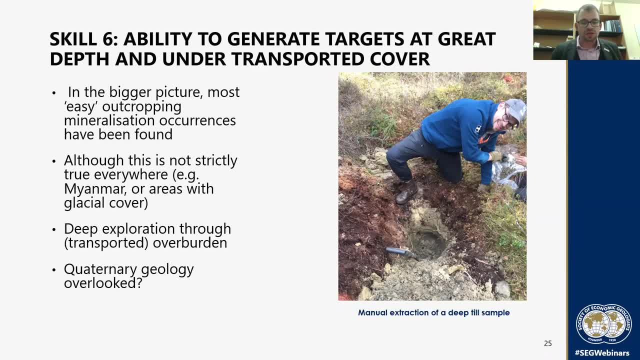 I recollect, I recall a situation where I walked over an outcropping, a 10 meter wide outcrop of massive lead sink mineralization, and this mineralization extended for kilometers along structural features or fault zones In northern Europe, in Scandinavia, the only problem you have is the till right. 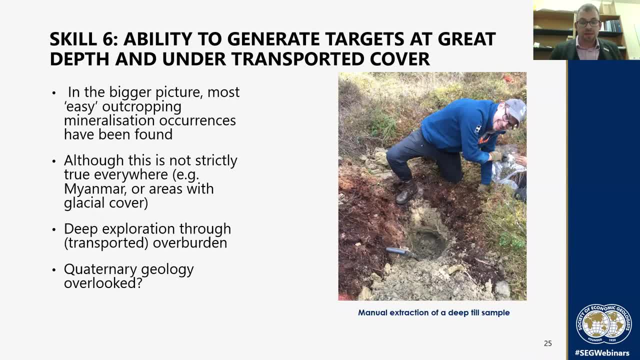 can be up to 10 meters thick, but then gold mineralization can be quite shallow, so we're not talking hundreds of meters deep And anyway, the ability to generate target through possibly transported overburden is very important. So the question here is: is quaternary geology, so quaternary land? 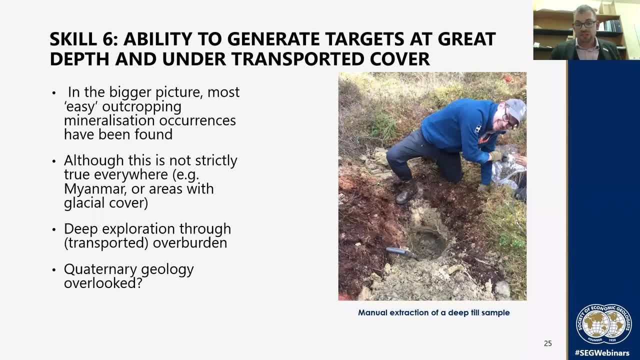 forms that have been produced by the recent glacial action. is quaternary geology actually overlooked? I believe it is Because it's not commonly talked. taught at universities, depending on where you study, and not really a big significance has been put onto it. but really understanding these transportation processes and secondary 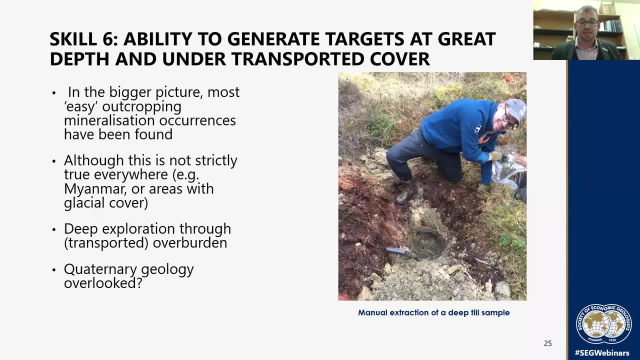 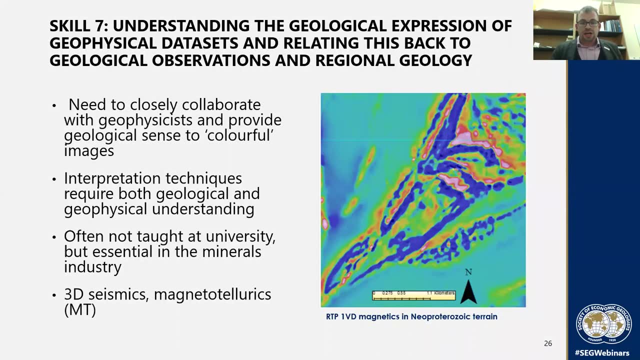 dispersion processes of overburdened material is absolute key in understanding where your soil anomalies are coming from. Okay, so let's move on to skill number seven. And skill number seven is the understanding of the geological expression of geophysical data sets and then relating this knowledge back to geological observations and regional 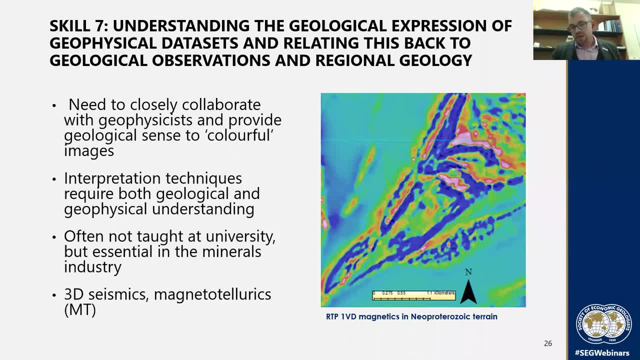 geology. On that figure on the right hand side you can see an excerpt of an airborne magnetic survey. It's actually one of the best Airborne data sets I personally have worked on And you see here the already filtered, reduced to pole first vertical derivative filter of: 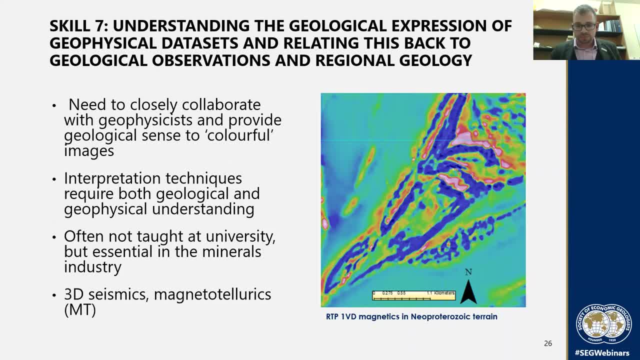 an area of this airborne survey And really geophysicists who collect and process the data. they deliver such images to the geologist Now understanding what these images, these red and blue blobs, mean. this is really important for us geologists because such data sets help us in understanding the geology and the mineralization. 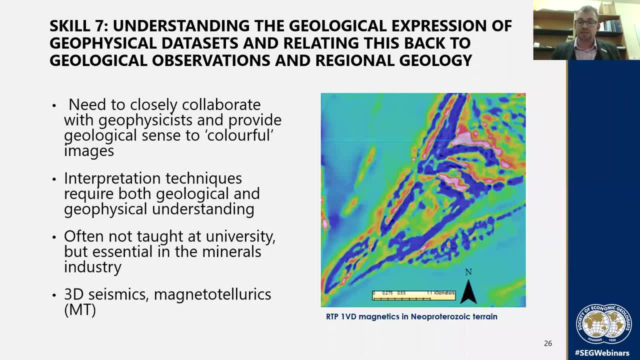 a lot better and in a way, help us to identify and establish a control on the mineralization system. In this image, for example, you can see or distinguish- You can distinguish at least two deformational phases. There's one deformational phase which produced a fold, and there's another deformational 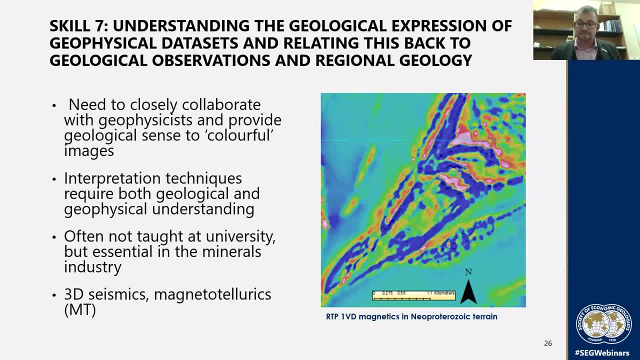 phase which is actually reflecting a sinistral shear zone here And it offsets the one limb of that fold to the west here. Maybe if you take a bit of a closer look at that you hopefully will see what I'm talking about here. 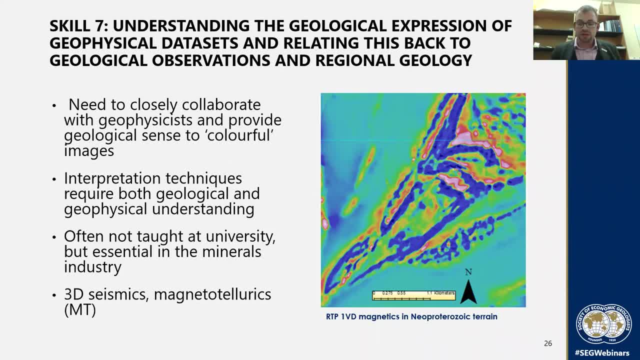 But this, of course, is of key importance. if you're looking for structurally-hosted ore deposits, such as orogenic gold or sedimentary-hosted copper, You want to identify where are the key structural features in an area and how are they related. 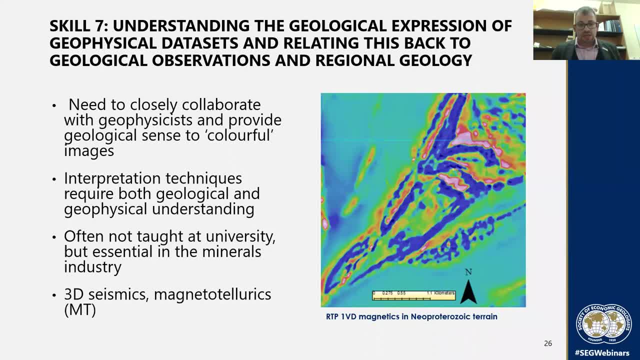 to mineralization. Now such interpretation techniques. first of all, they're often not taught at university right, And very often people pick up these skills by either mentoring, that a more experienced geologist is teaching them, teaching younger geologists how to interpret such data sets. 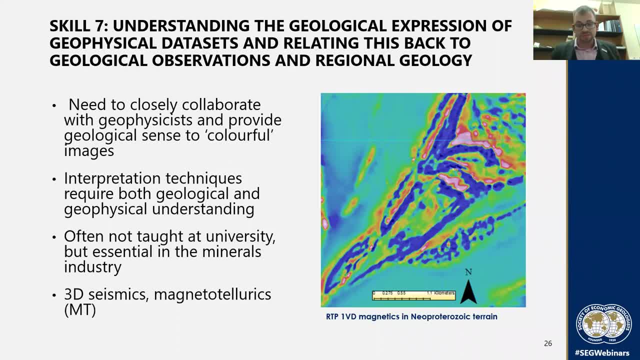 or they learn it by doing or attend workshops, but really, from what I see around, this skill needs a bit more, Yeah, attention in university curricula. Importantly also is that geologists need to communicate to the geophysicists, who can explain. 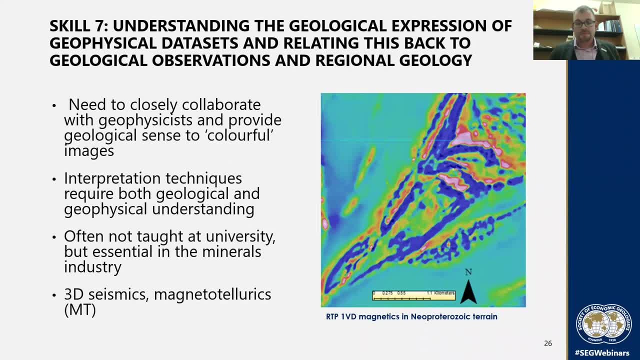 what these different mathematical derivations of the data set and the resulting colors actually mean. So you know, if you ask a geologist, what is reduced to pole first, vertical derivative geologists probably have struggled to understand the mathematics behind it. That's why it's important, if you know a geophysicist who can explain you this in great detail, that 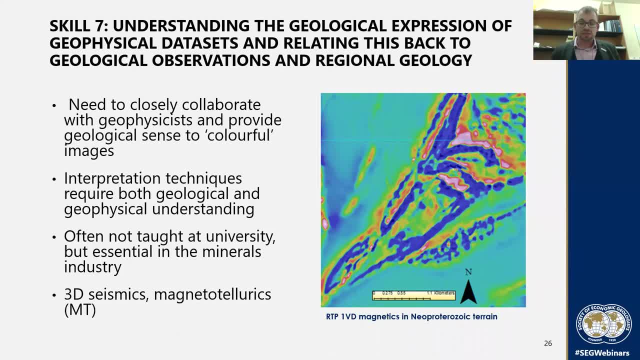 you learn from our colleagues in geophysics and use this knowledge and these skills to fine-tune your structural interpretation, for example. A few other key techniques that have really, Yeah, become important in mining are 3D seismics and magnetotellurics. 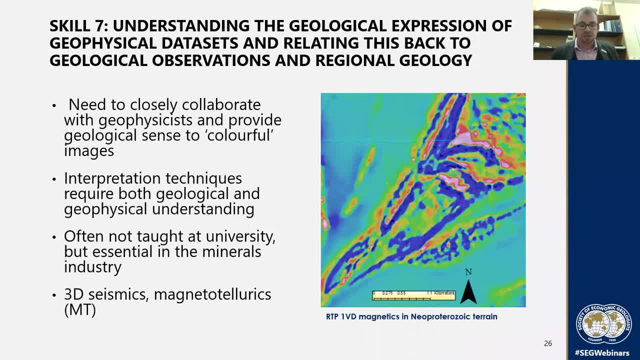 Now, 3D seismics has been on the oil and gas market for an extremely long time, but mining industry- we are currently waking up to the idea that 3D seismics could be interesting, especially if you study sedimentary or metamorphosed sedimentary basins. 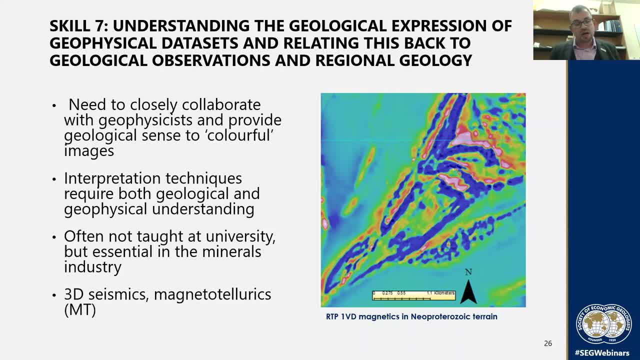 Magnetotellurics. Magnetotellurics is a very useful tool. It's been around for a long time as well, but it's also in the last decade. people have realized the use of it when exploring for deep deposits. 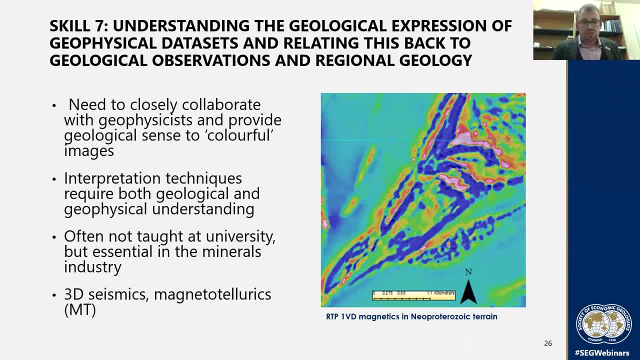 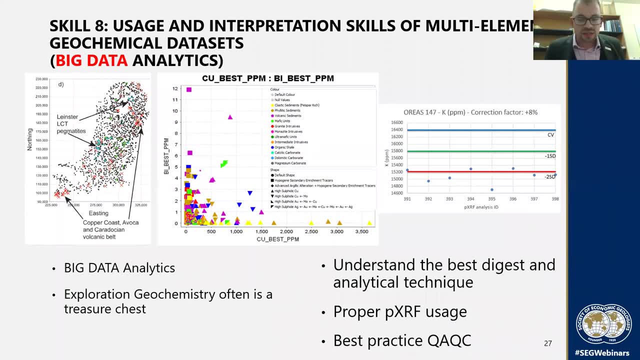 Okay, let's move on to the next skill, skill number eight, And this is all about big data analytics. You may have heard about artificial intelligence. Okay, This is all about big data squeezing and all these data challenges that have been around over the last couple of years. 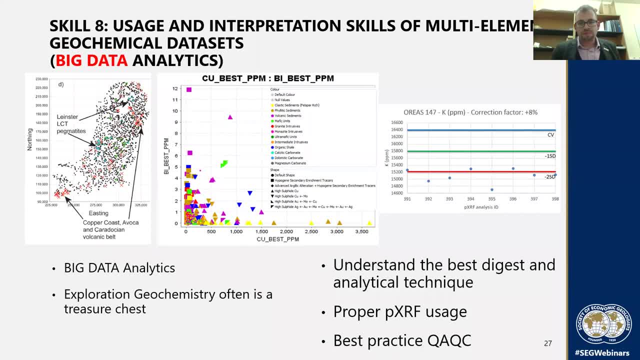 During PDAC over the last few years, there were always The winners of these big data. challenges have been presented And nowadays we have or mining companies or governments. they've accumulated huge amounts of data, may it be geophysical or geochemical. 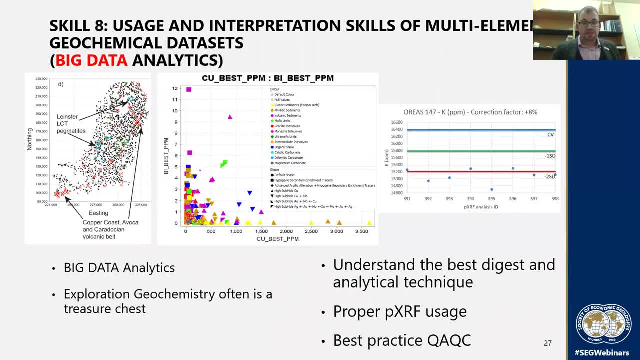 Huge data sets are available out there, but here it is important to be able to know what to do with such big data sets. right? How can we extract useful information from, for example, large-scale geochemical data sets? Now, nowadays you have all these sophisticated techniques such as geoscience, geoscience. 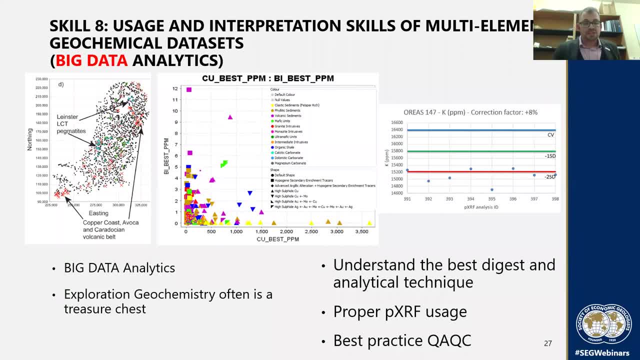 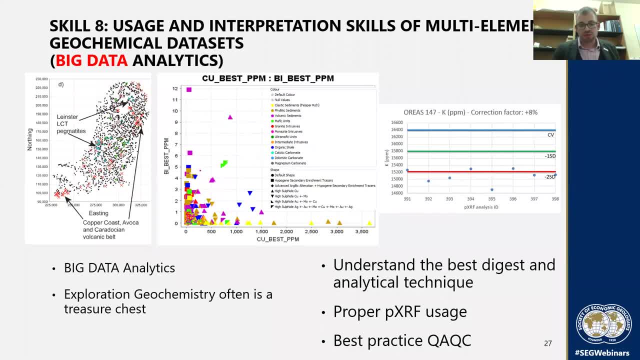 Just to name a few of these buzzwords. they really become important in the very near future, So knowing about these skills is key, So I put up a few images here for you to illustrate how important it is to understand your- in this case, geochemical- data. 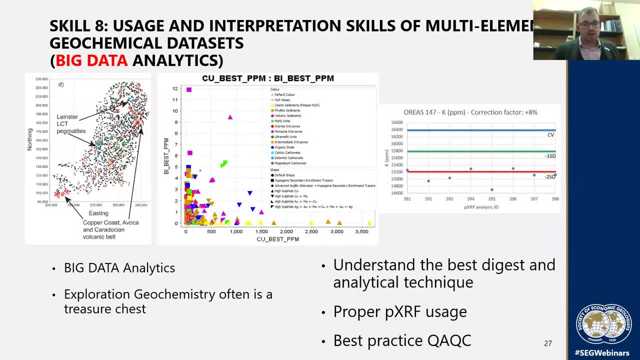 On the left-hand side you have a map of Southeast Ireland in Europe And this area has been, over the decades, sampled extensively. You've got lots of stream sediment locations here. I think this data set contains something like 5,000 data points. 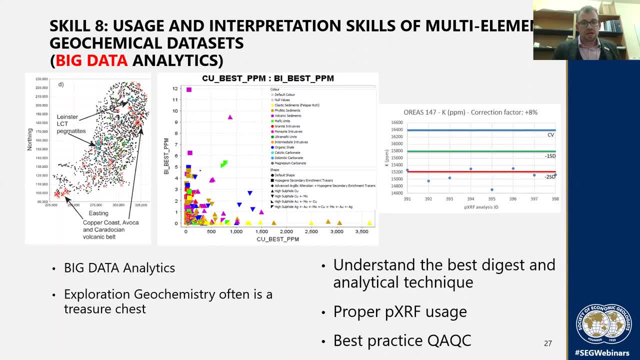 Now being able to extract key information from this data set. Therefore, we have to pinpoint where occurrences of mineralisation are very important. So very often, exploration geochemistry is a trestle chest. You just need to know how to open this chest. 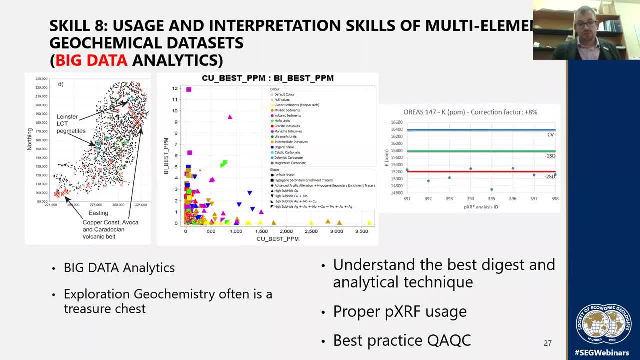 You know, you need to know the tools to, to apply and squeeze this data. That figure in the middle, Ms, Here on the right hand side. l is, l is now a, what L now l is live existent. 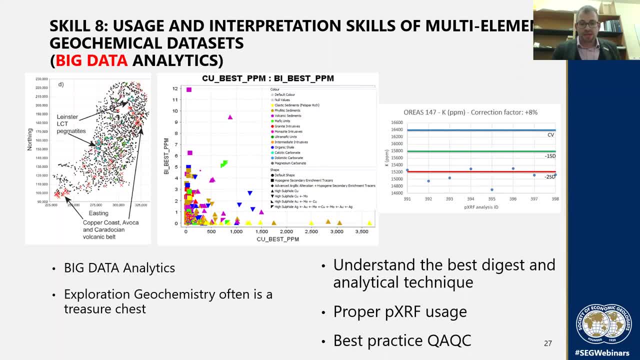 open source data set from British Columbia, I think. it contains about 15 or 16 thousand data points, an incredible amount of data. And here I try to understand: how can we extract from this cloud of data any meaningful trends that could lead us towards a discovery of porphyry copper deposits? Now, this is 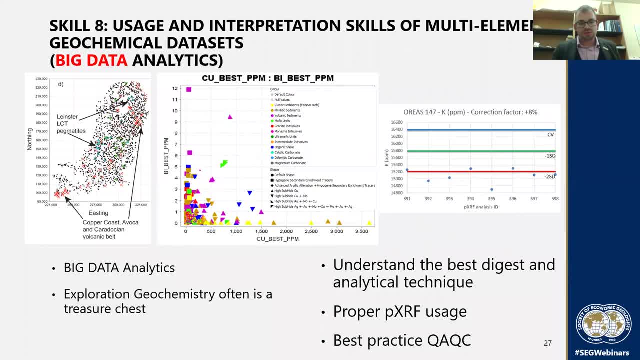 just one graph here that was produced. there's a lot more going on there and during that study, but if you understand how elements work in mineralization systems and what they indicate, such as in porphyry copper systems, if you identify the elements that are typical for advanced 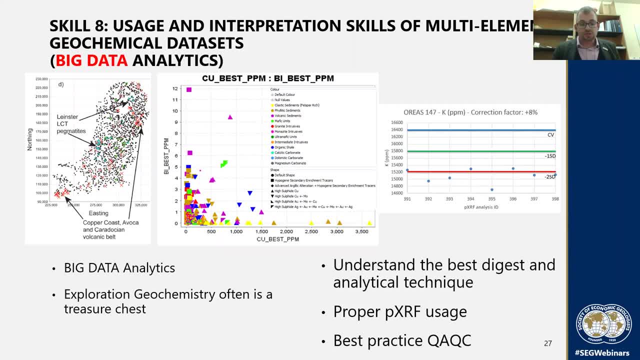 algeolic alteration or hypergene secondary enrichment of elements, then these elements will be produced in a similar manner. But if you elements, that will really help you to understand the occurrence of potentially blind porphyry deposits. And on the right hand side you see a quality control chart of certified reference material. 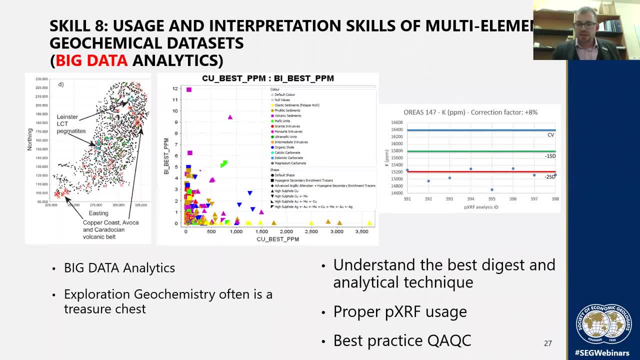 that was analyzed by Portable XRF. Of course, all the data that I'm showing you here, all of these tens of thousands of data points, we need to ensure that the quality of it is acceptable. So we need to ensure that the data is telling us something meaningful and it's not just. 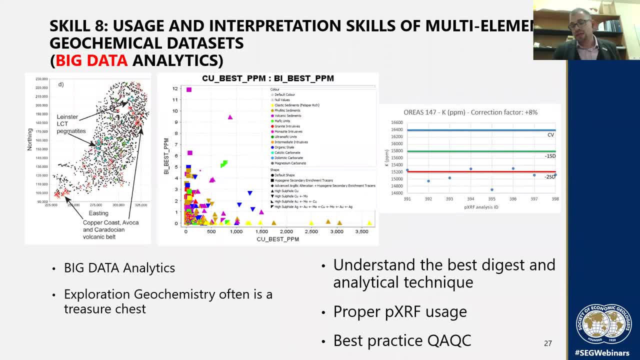 any collection of random numbers, And for that often, well, that's a must. in fact, you need to apply quality control procedures by a applying certified reference materials, and so on. Now, as a geologist, you definitely have to understand when an analytical technique is. 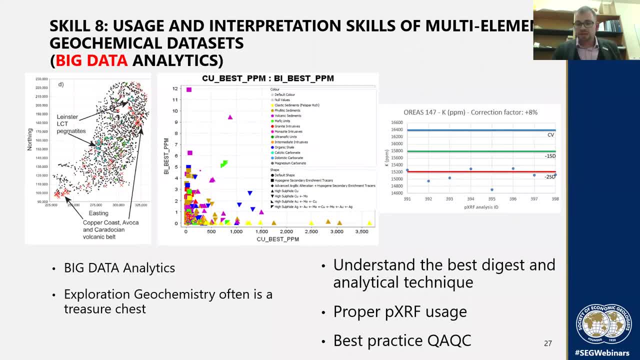 not working properly. For example, here in this graph on the right you can see that that's the potassium values on that PXRF. that Portable XRF that was in use is really quite underestimating the certified reference material by about 1500 ppm or so. 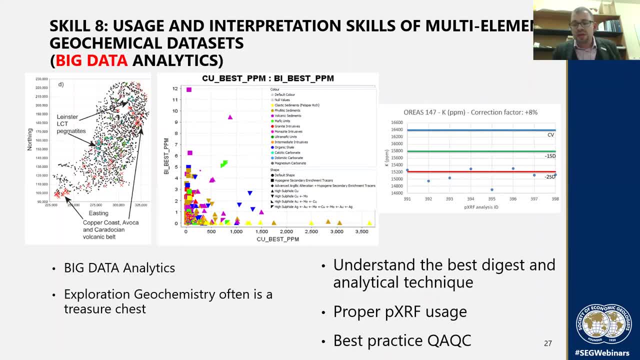 Now you need to recognize this as a geologist, because if something similar happens for your mineralization suite, then you might well underestimate the potential mineralization that is there and available. Okay, so best practice, quality control is very much important If you deal with such big data analytics. 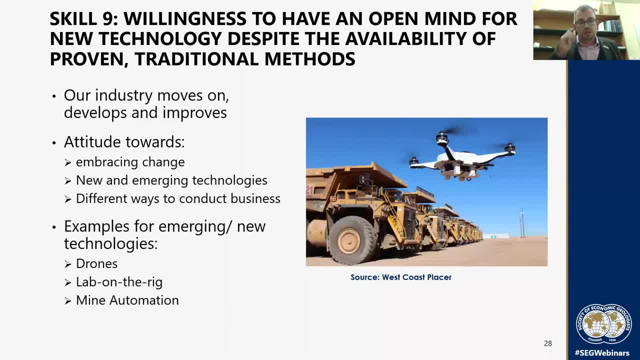 Okay, moving on to the next slide, I believe that the that you should think about the willingness to have an open mind for new technology despite the availability of proven traditional methods, And The key point here is that our industry, the mining industry, moves on. the industry develops. 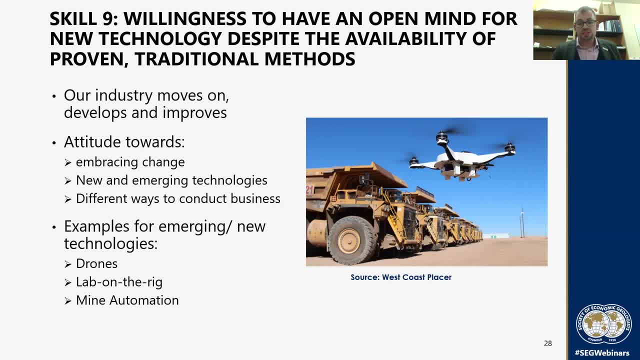 and it improves, So techniques that have been successfully used 50 years ago that might still be valid nowadays. However, as technology improves, there are better technologies coming out nowadays that can really help us to to gain the cutting edge on our mining and and, and you know. 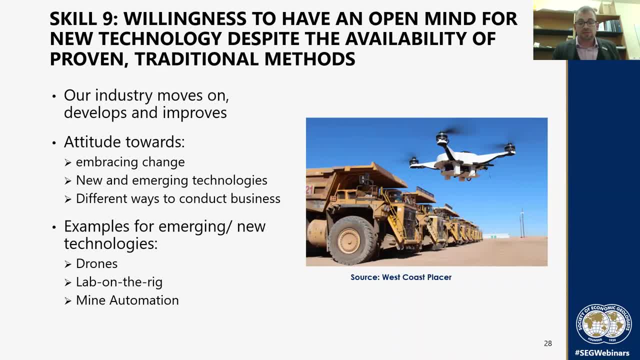 exploration, exploration. So developing an attitude towards change, not being resistant to change and embracing these new ideas and technologies is very important, right And, for example, key things that drive our industry nowadays are, for example, drones. Drones really have picked up in the last five to 10 years. 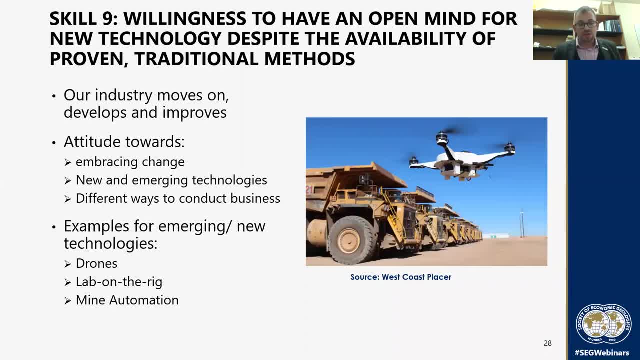 And nowadays it's very common actually that you can. you can mount a magnetometer onto a drone, like you see on the right hand side, And whilst in the past, airborne magnetic surveys, you know, were conducted at quite wide spacing between the sample lines, it's not uncommon that if you've got a flat area that you fly. 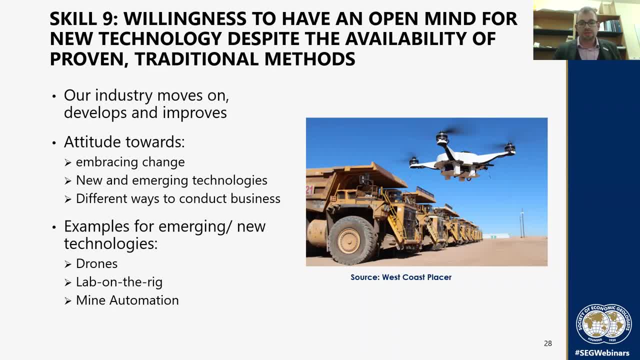 a drone at 10 meters altitude and 10 meters sample line spacing. That really will give you an exceptionally an exceptional data set that can be used. So I think you should watch the space, and it's maybe not not a bad idea to if you. 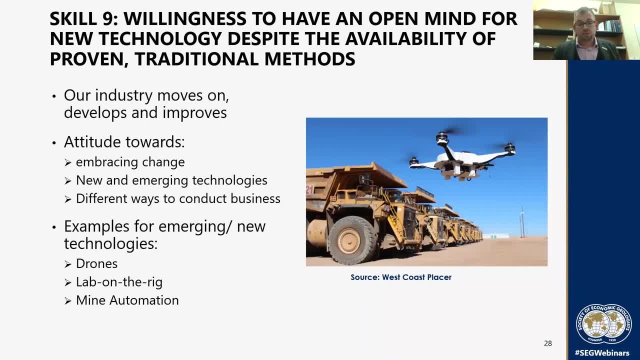 have the chance to to maybe get a drone driving license so that you can officially and legally drive drones or fly drones, and perhaps they can become important in your job later on. A few other technologies that are currently being developed is the so-called lab on the. 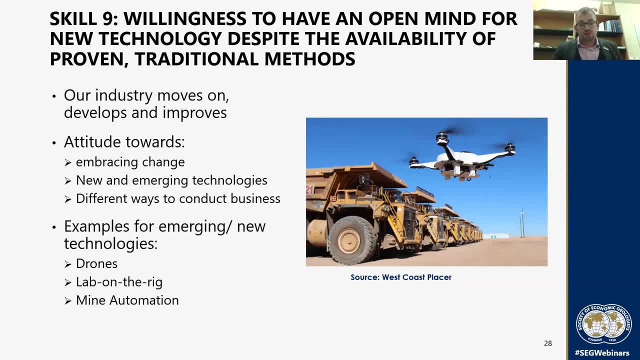 rig. So traditionally you drill a borehole, you extract the sample, maybe have a portable XRF that you use to quickly sap over the samples and determine the content of metals in there, And then it's been usually sent off to a lab. 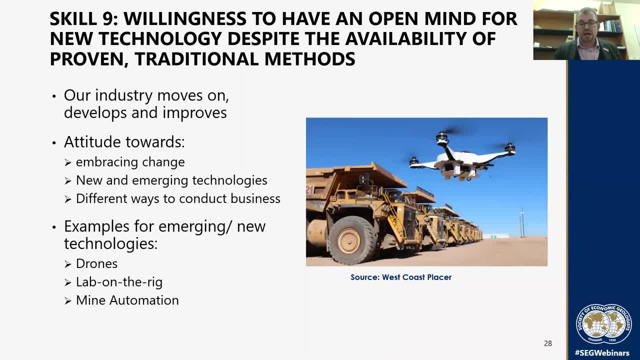 Yeah, That's a commercial lab somewhere else. I will really. nowadays, people are developing and companies are developing the so-called lab on the rig system, which allows a really fast turnaround of samples on your work site, And this is, of course, very important implications for the turnaround of samples and for the 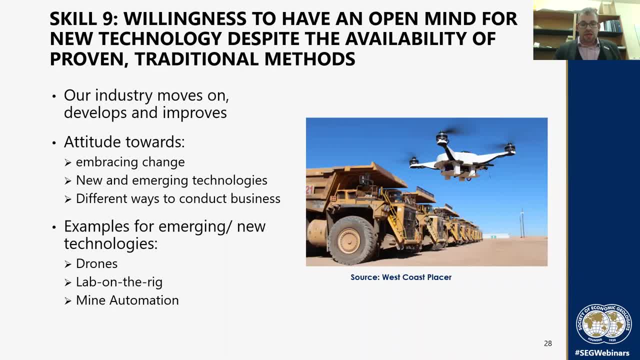 ability to make decisions very quickly. Okay, Thank you. And the last point here about mine automation. you may have seen these videos of the big mining giants in West Australia where they sit in an office in Perth and they are driving trucks remotely a couple of thousand kilometers away using remote equipment. 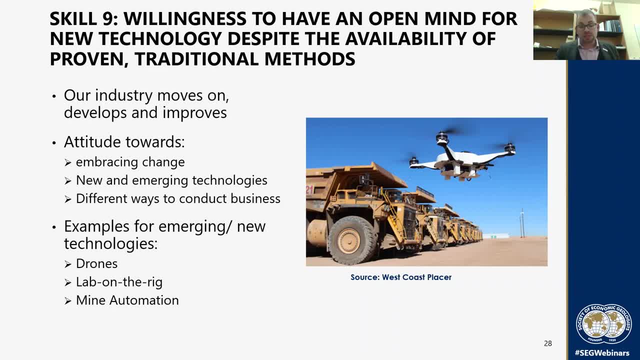 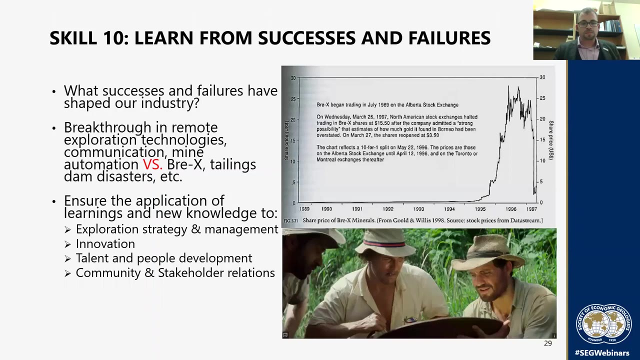 Now that is just a starter into the mine automation direction. Maybe it's, perhaps more important for mining engineers, but definitely one of the key new technologies or areas of new technologies that is currently being developed. Moving on to the next slide, I guess, to wrap the top 10 skills off, I believe it is also. 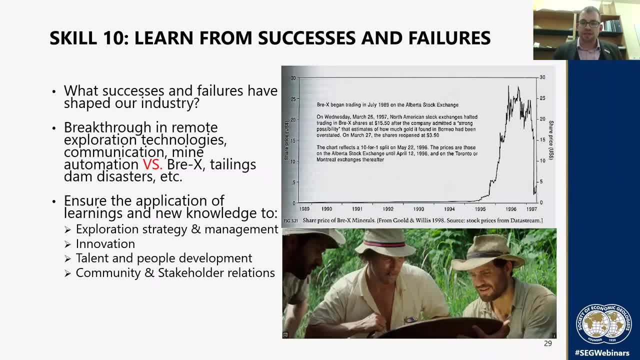 important that we learn from successes and failures. Yeah Yeah, There have been many different successes and failures in our industry- mining- and we need to learn from those. I mean probably one of the classic failures over the last two or three decades definitely. 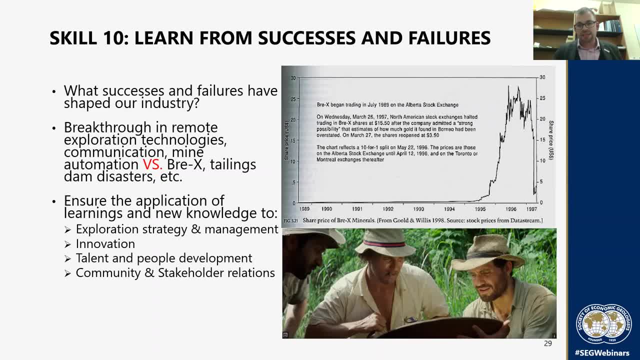 has been this so-called pre-X situation. Maybe you've watched a few years ago in cinemas the movie Gold, pictured on the bottom, which is basically displaying this event. that happened in the 90s in Asia, where investors and geologists have misled the stock exchange and other investors into believing mineral deposit was of great 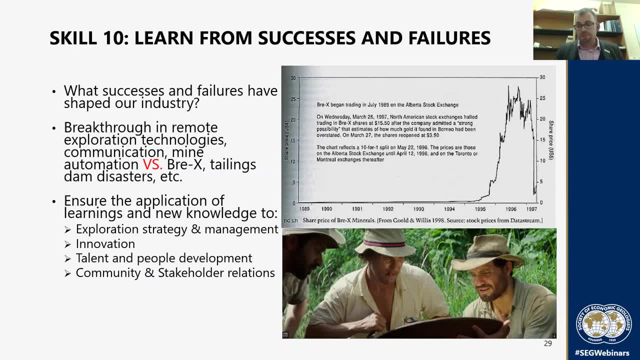 value And that, of course, boosted the share price considerably, Only to turn out That it was all fake and all fraud actually, And that event led then subsequently to a strict implementation of these resource reporting codes, in the hope that such events are minimized or do not happen in future again. 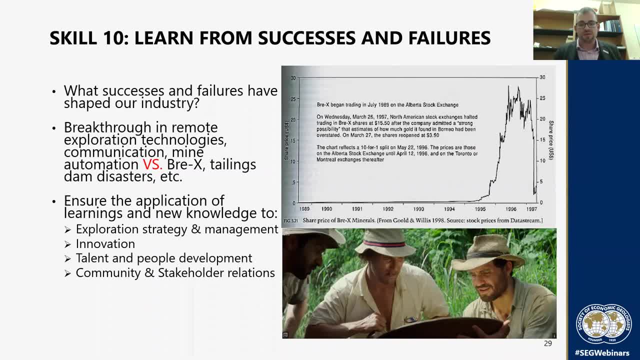 Now this pre-X is one of the classic examples of a failure recently. However, that needs to be seen against All the successes we have also in the mining industry, such as remote exploration technologies, mine automation that I mentioned just earlier. So it's good to be able to read into such case studies of good and bad aspects or developments. 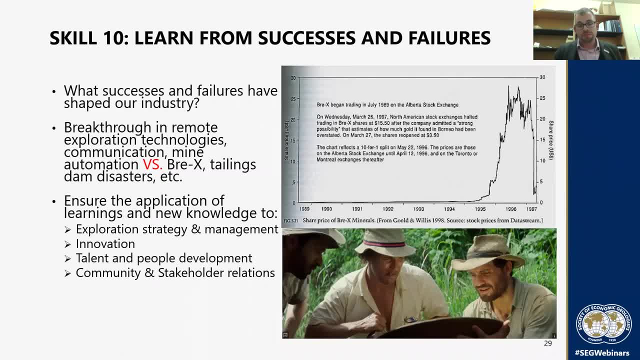 that have happened and learn from those. We want to not repeat the same failures that we've experienced in the past. Yeah, So We really need to ensure the application of these learnings And we need to think about how do we run our exploration programs. 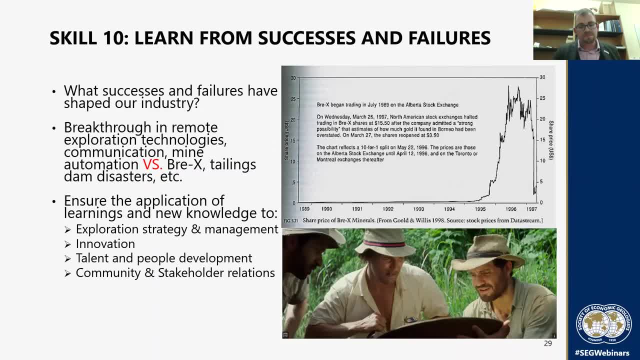 How can we redefine and streamline the strategy to drive and develop projects, And also that you need to consider innovation, Talent and people development. all of these aspects are running into this: learning from successes and failures. All right, So I think we have another, another yeah poll coming up. sorry, I lost the verse here. 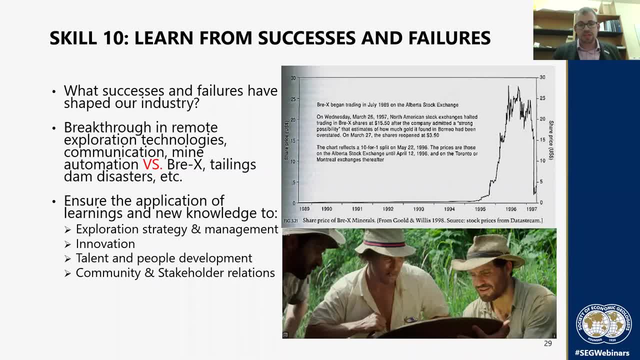 Before we move on to how we acquire these skills, I would like to ask you: how do you think you acquire new job relevant skills? Are you studying advanced degrees like masters or PhD degrees? Are you attending presentations at conferences and seminars? Are you attending networking events and learn from other people, or do you just learn by? 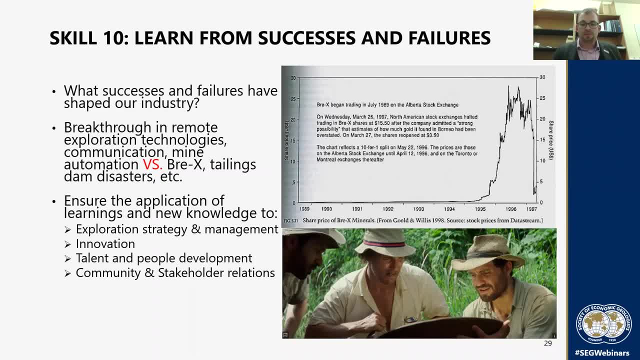 carrying out a job, in doing your daily work. So please choose one of these options And let's take a look. Let's look at how you guys believe you can acquire new skills. Okay, I've made my choice here. Let's wait a few more seconds. 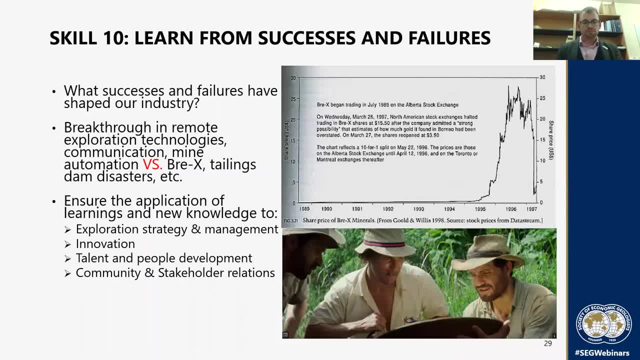 All right, Thank you. Thank you All right, Deanne. if you would like to share the results of this poll here, Excellent, Okay, So we have a clear winner here: 56% of you believe that job relevant skills can be actually learned on the job. 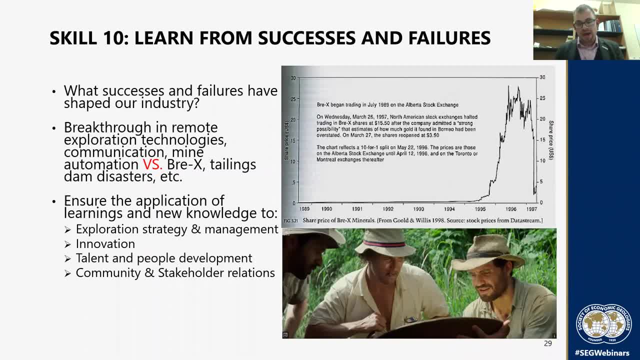 So, for example, you're running a project in the Outback and someone asked you to investigate logistical or procurement issues. solve them. You learn it on the job. Well, I think that's a very valid view. We've also got some other opinions here. 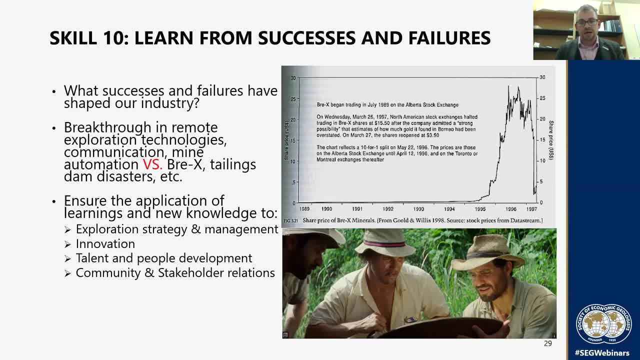 People like to attend presentations at conferences or attend workshops, learn from experts in their field about certain techniques and studying advanced degrees. Yeah, All very relevant. So thank you very much for this poll. And let me quickly- And I appreciate we're running slightly over time- 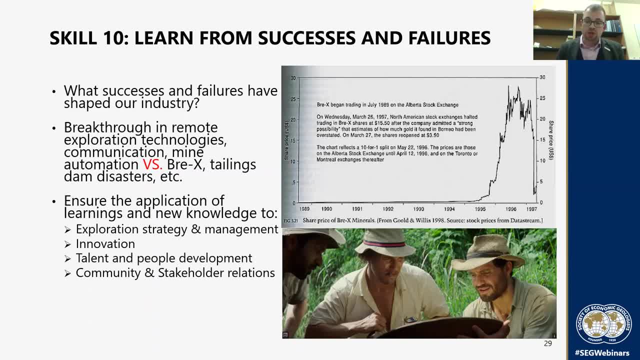 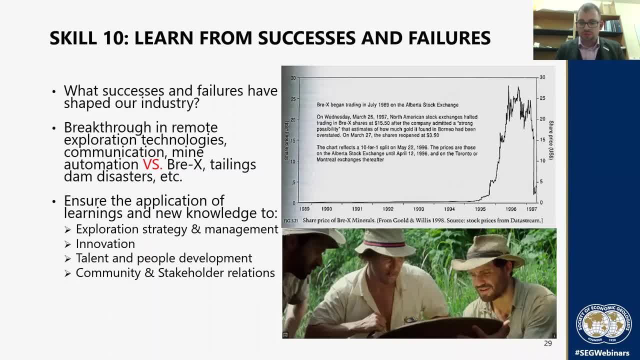 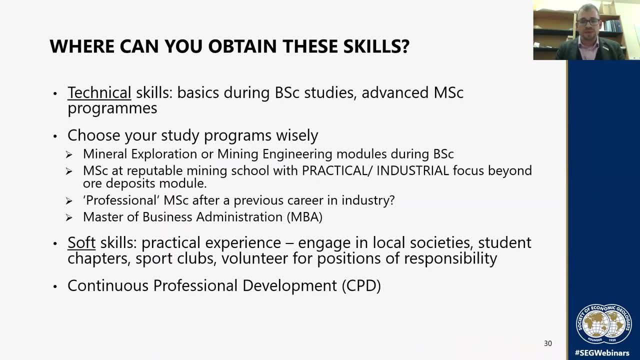 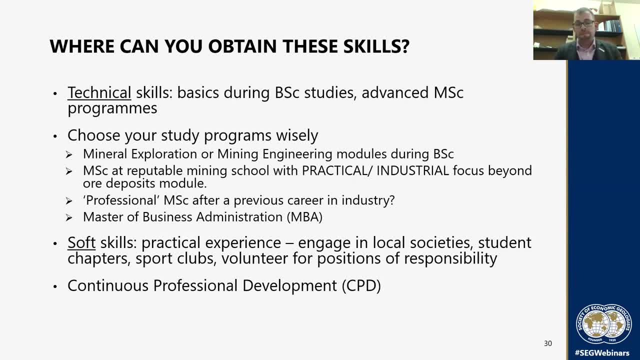 number one. these basics really there should be. you should learn them during your bachelor's studies, your undergraduate studies, such as rock identification. a bit about all the possibilities. Okay, Thank you. Okay, geology, perhaps, and mineral identification: Really then advanced. 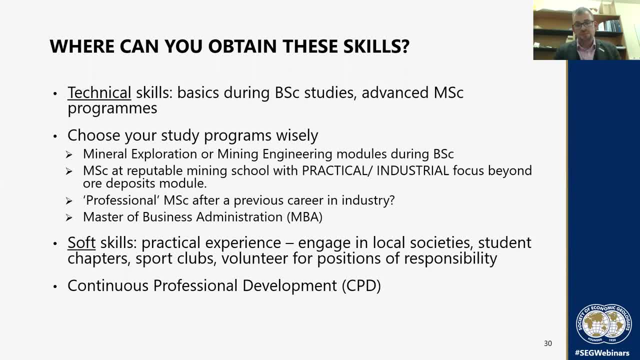 master's programs are usually a very smart way of getting the specialist skills that you need for your job. That's why we have advanced master's programs around the world. My recommendation for you if you're at this stage is to choose your study programs wisely During your undergraduate study, if possible. I 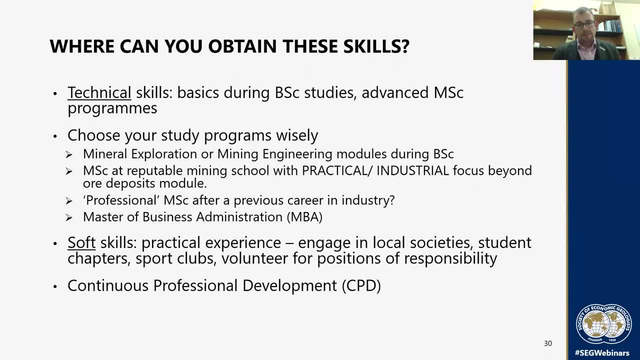 recommend you to attend mineral exploration or even mining engineering modules so to get a broad overview of the techniques that are used in the mining industry. If you do a master's, either after your undergraduate, or if you come back from university, from industry down there, you see a. 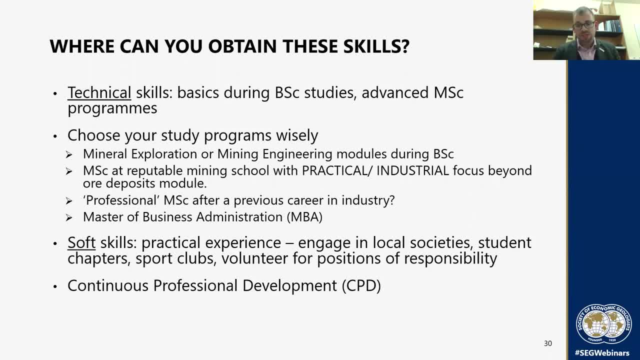 professional master's. so if you have a couple of years experience and come back, My strong recommendation is you need to do this at a reputable mining school with- in bold letters, a practical or industrial focus beyond the usual ore deposits module. Many universities offer ore deposit module where you learn about how. 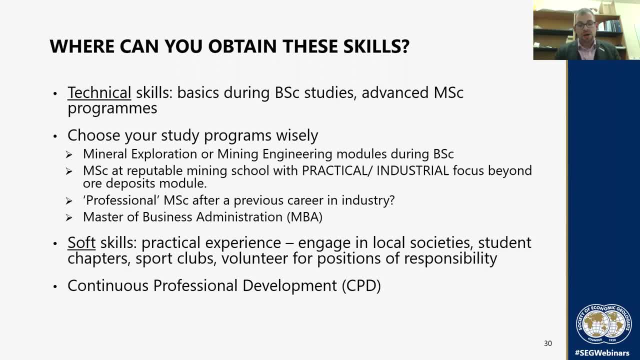 different deposits form, how you can study them by optical photography. I think that's what one person mentioned earlier. Now that's the standard, but really it does not necessarily cover the skills that you need when you're out in the bush and trying to find an ore deposit. So, please, 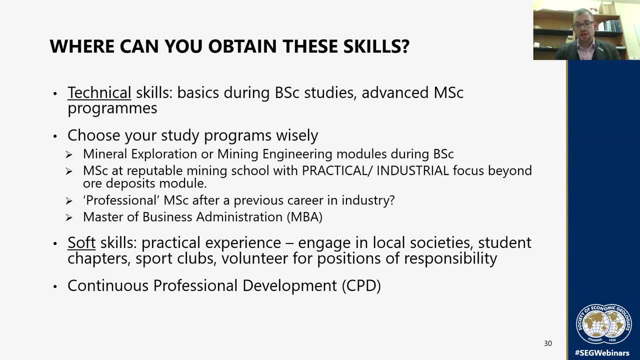 my recommendation: if you choose advanced study, try and look for the mining schools which have tailored program and cover all the techniques you need in geochemistry, geophysics, site investigation and so on. It is also a very good idea that if you spend 5,, 10,, 15 years in the industry, 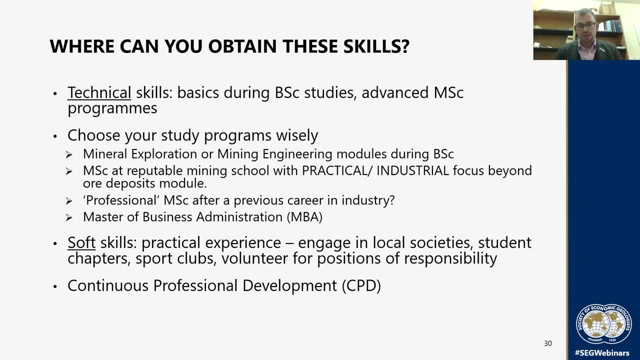 and you would like to return to do a master's. that's not a bad idea, And I know several people who do this to boost their skills in a specialist area, And mostly these people have a clear idea of what they want from the study. 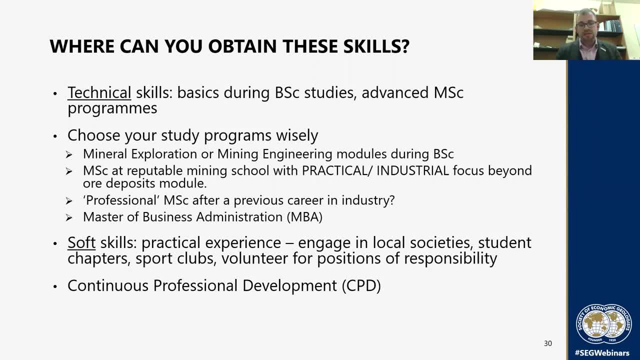 So they've done their 5 or 10 years in industry and they know exactly where they need to improve their skills and that's how they target to get this formal education. If you're thinking of moving into a more managing role, like becoming an exploration manager or director. 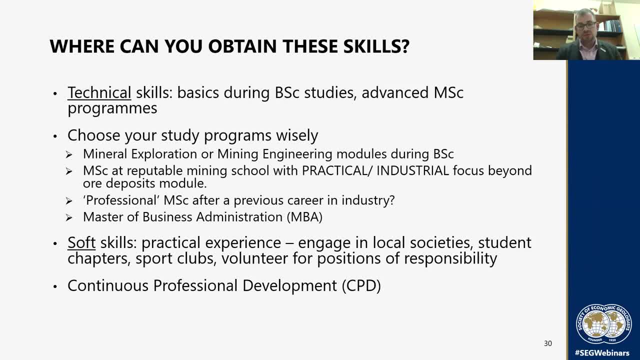 it's also great if you consider doing a master's of business administration, Because this will allow you to gain skills on marketing, on setting up companies, on finance, and they are usually tailored to industrial projects and career paths. The soft skills, on the other hand, these are what you usually do. 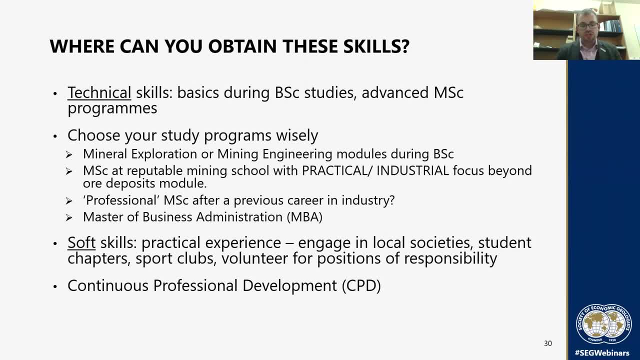 They do not learn at university. Remember the logistical, the health and safety or the community skills. This is really practical experience that you need to gather on the job, And mostly students who seek these soft skills. I recommend you engage in local societies- student chapters. 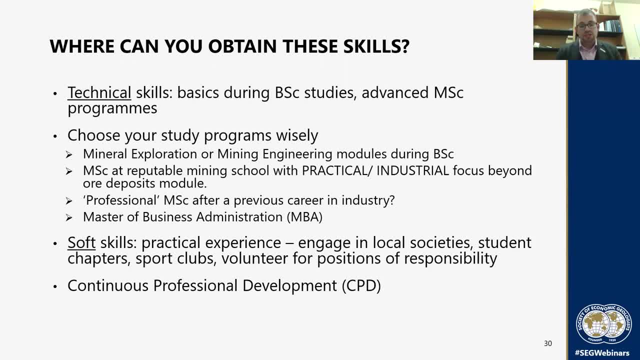 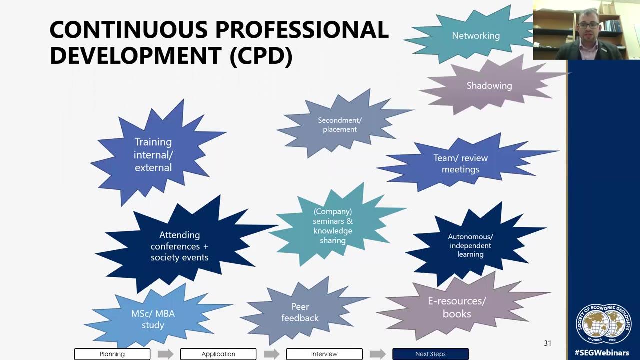 We've heard earlier from Deanne that the SEG is running 118 student chapters. You can engage in sport clubs or volunteer for positions of responsibility. This exactly will improve your management and your leadership skills, And for the professionals amongst us. let me move on to the last slide about continuous professional development. 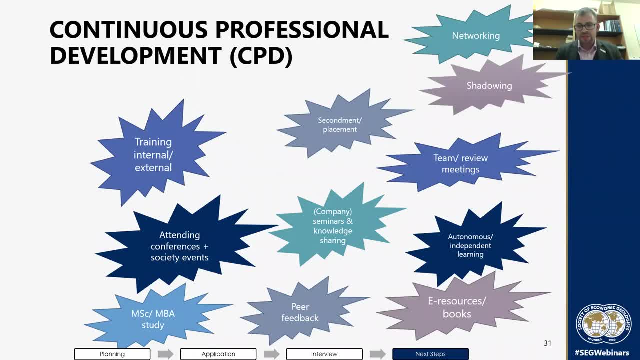 I think I showed this last time as well, And really when I started off my career in mining, I thought that The only way I can develop is by attending expensive workshops and courses. That's what I thought at the beginning would be how I learn new skills. 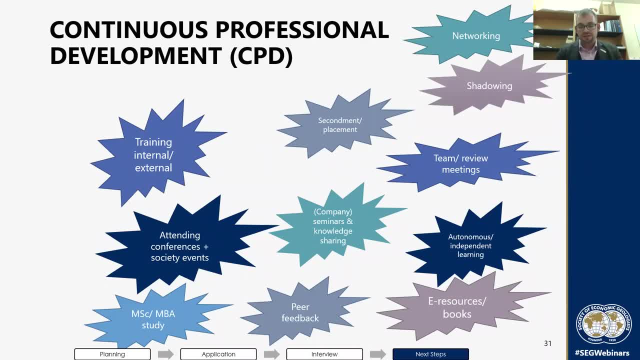 But actually time has taught me differently and is really a range of activities you can do to improve your CPD, your continuous professional development, Whether that is participating in team meetings and presenting your results to the wider team or to management, or whether you can get a secondment or placement to a mine site or to another project, to another country for a couple of months. 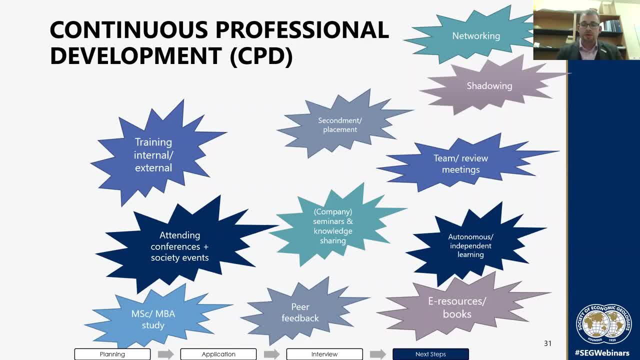 It could be that you shadow a very experienced person in your organization and you learn about, you know how experienced people can be, How experienced people can carry out their jobs. That is really valuable. I believe You could attend networking events or in some parts of the world they're called mining sundowners. 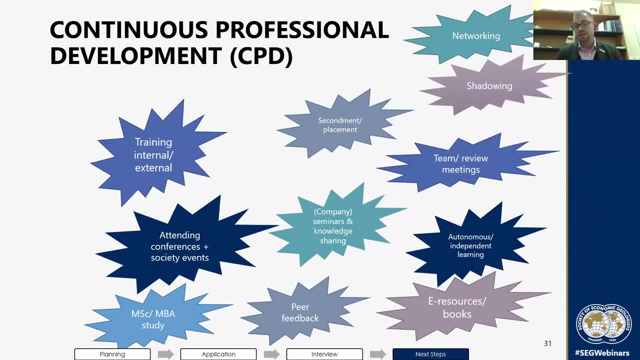 where people meet informally, chat about life, chat about developments, And you can learn a lot from people attending these events. You may want to consider attending conferences or society events. Just last Last week, we had the SEG annual meeting in Santiago. 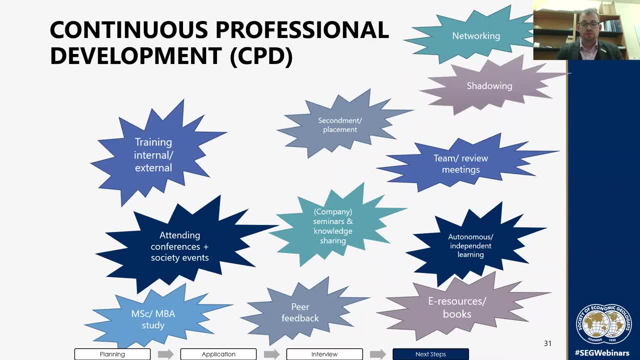 I couldn't attend myself personally, but this is, of course, if you manage to attend. it's a great event with many different participants which allow you to listen to state of the art science talks and network with people. So all of these aspects here on the slides are really forming your CPD. 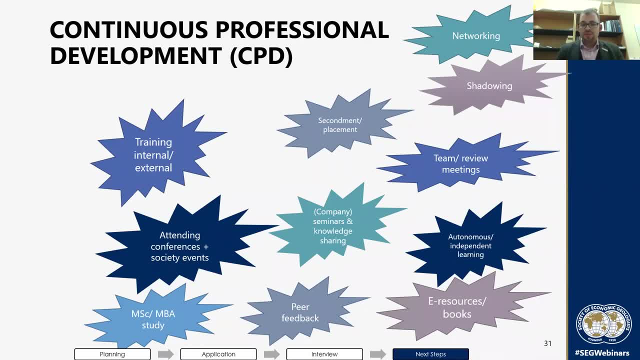 And very often in your professional development. if you're a registered geologist or a chartered geologist- or in North America it's a professional geologist- you need to maintain a record of your professional development, And those are just ideas how you can boost up your CPD beyond simply attending any workshops or courses and listening to people. 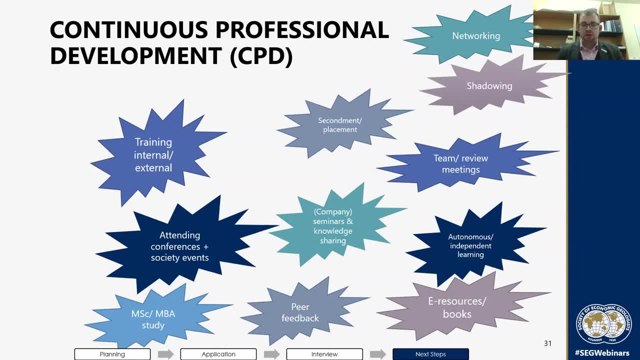 Okay, so this slide, of course, will be available. So if you have any questions, please feel free to reach out to me. I'll answer them all later on And please feel free to consider some of these aspects presented here. Great, 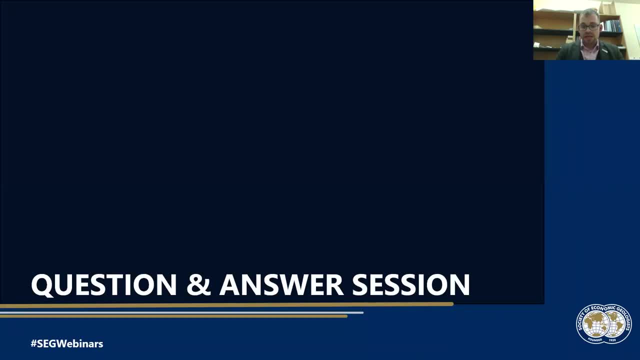 I think this was the last slide. Let's move on to a question and answer session. We have a number of questions here, And let me Quite a few. actually, Let me go through, Let me find, Let me find one that I can answer quickly. 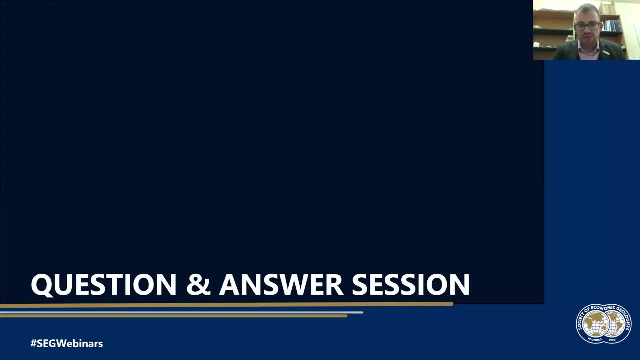 What skills does a PhD student need to have at the end of his PhD to work in mining companies? Well, quite often, as a PhD student or someone with a PhD degree, you are regarded as a specialist person, having studied a topic in great detail for a number of years. 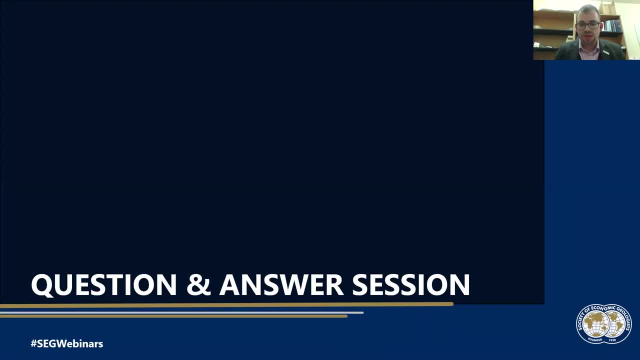 So here I would suggest that you try to show or demonstrate experience in a number of aspects that are unrelated to your area of PhD study. Okay, so if your PhD was on- I don't know- nickel, copper, PGEs, maybe you want to present skills that show a wider spectrum of understanding of the minerals industry, of exploration techniques and of. Okay, so if you're a PhD student, you want to present skills that show a wider spectrum of understanding of the minerals industry, of exploration techniques and of. Okay, so if your PhD was on I don't know- nickel, copper, PGEs, maybe you want to present skills that show a wider spectrum of understanding of the minerals industry, of exploration techniques and of. 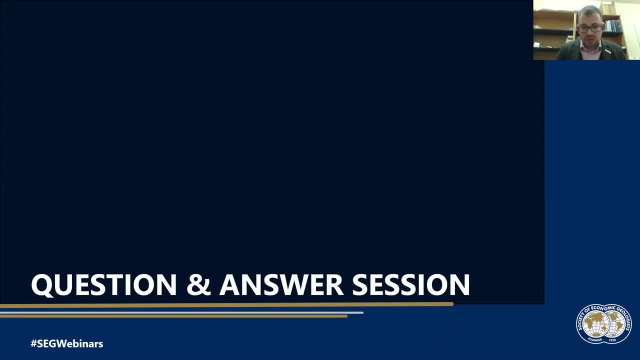 Yeah, how to evaluate all the? Let me move on to the next question. Well, here is one. At which frequencies do you analyze seismic information? I'm afraid I cannot answer this one. I'm not a seismic interpreter. Sorry, I can't answer that. 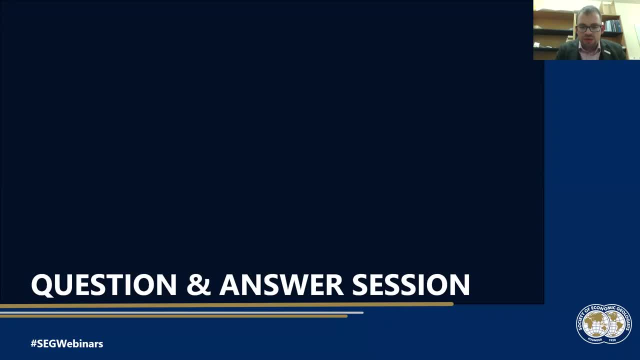 How do you think an academic and research, How do you think an academic and research-based geologist could fit in a mining company? Well, there are a number of ways how you can fit into a large organization. For example, if you're a specialist in a certain area, you could become. 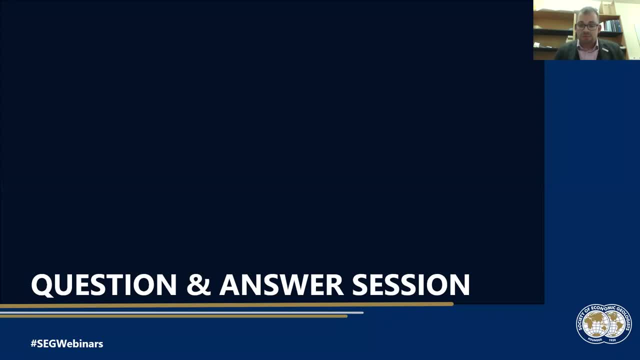 And you've got some experience, you could become- I don't know- a principal geologist in remote sensing techniques and really drive this aspect of geoscience in a company. Let me go for another one. Yeah, an important comment here. 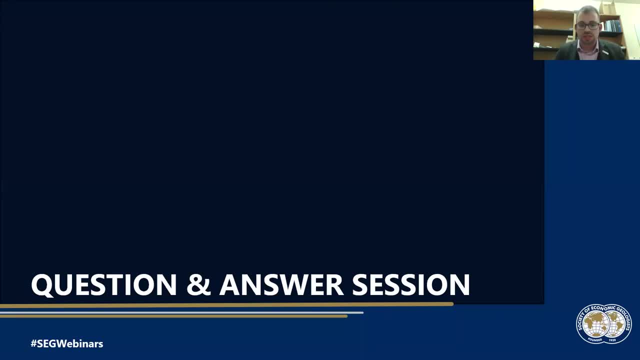 What about geological 3D modeling software skills? Is it still worth learning modeling? Yeah, thank you very much for mentioning this. I think I actually didn't have it in my slides, But this is exactly when it comes into big data analysis. 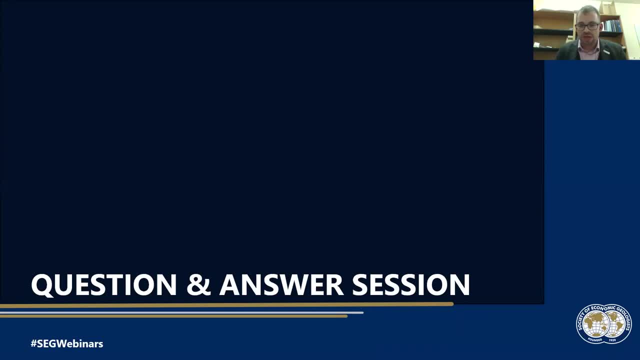 Of course it's important to learn about. you know how to produce 3D models, How to operate the software and, especially, how to know the advantages and pitfalls of such software that are currently used on mine sites. So, yes, definitely improving your skills here are key. 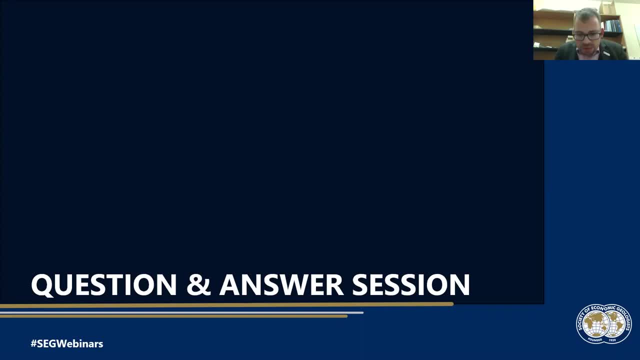 Another question is around. a geologist could be able to deal not only with technical knowledge but, more importantly, how important it is to develop management and soft skills. Absolutely, If you want to be around, if you want to be a showcase and demonstrate experience in many different areas. 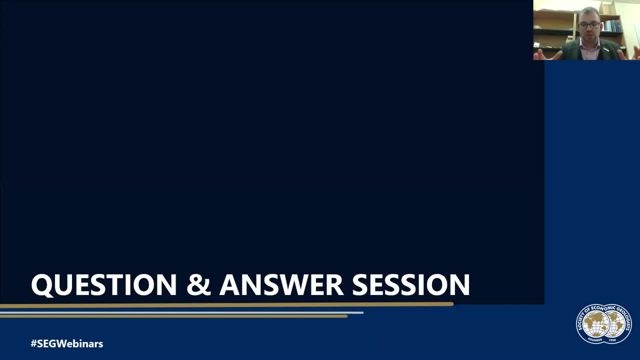 it's not just important to know your rocks, It's also important to deal with logistical soft skills and management skills. It's absolutely key. And the last question here: What is the most important thing for a geologist? What is the most important thing for a geologist? 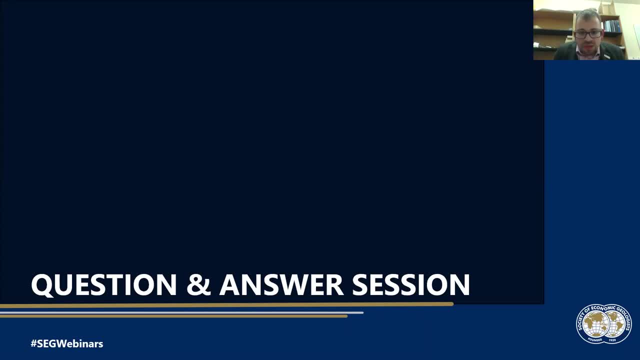 Are there any mentoring opportunities for geologists returning to the industry, For example, women who have taken time off to look after a family? I cannot comment this specific case, but I know that there are definitely in large organizations. there are mentoring opportunities where, as I said, like shadowing almost where more senior people look. 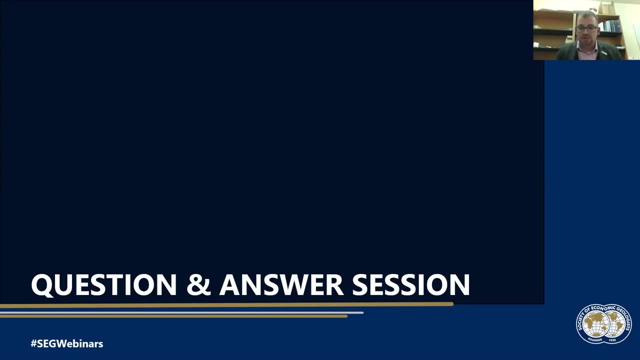 after you and allow you to, you know, to speak to them and you get their professional advice and direction, if you like, how to settle back into the job and how to advance. Excellent, OK, thank you very much for all these questions. 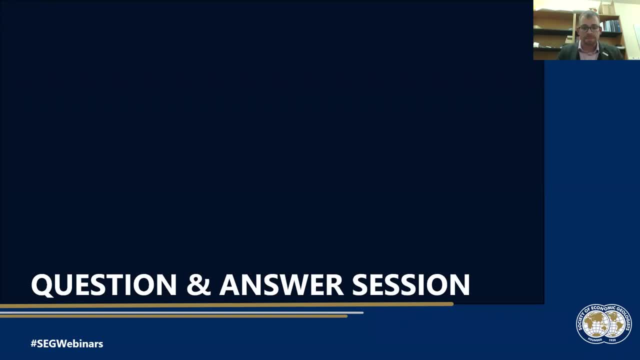 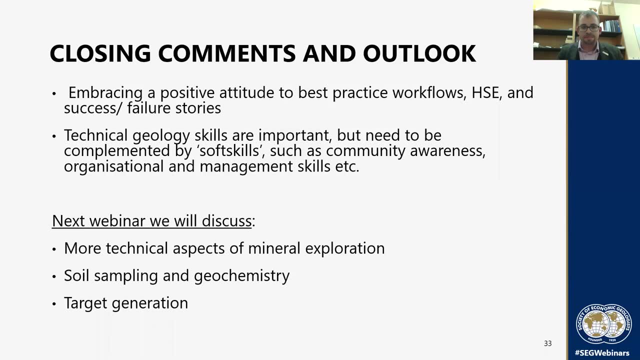 It's been really great to get such engagement from you guys. We shot slightly over time, so I think we should cancel it here, And I just wanted to let you know that during the next webinar we will really dive a bit deeper into the technical skills.